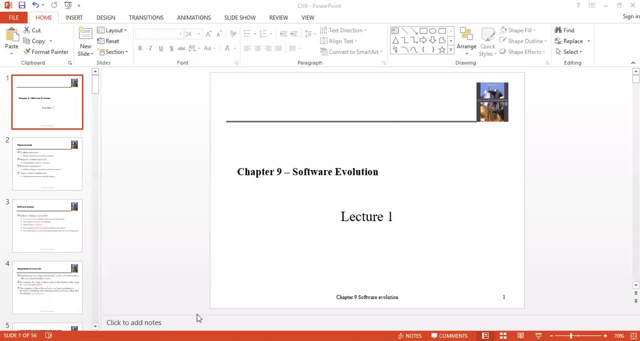 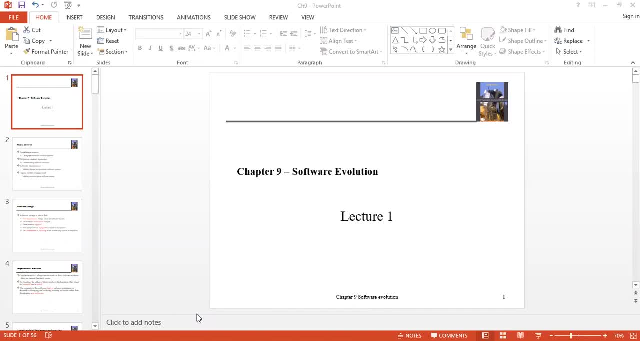 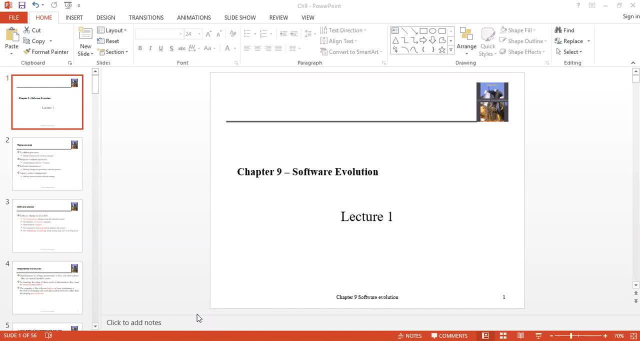 Assalamu alaikum, kids, Can you hear me? We have read its implementation and then we have read its testing and now we have come to its evolution. If we want to make any modification in our process, in our project, then we call it evolution. 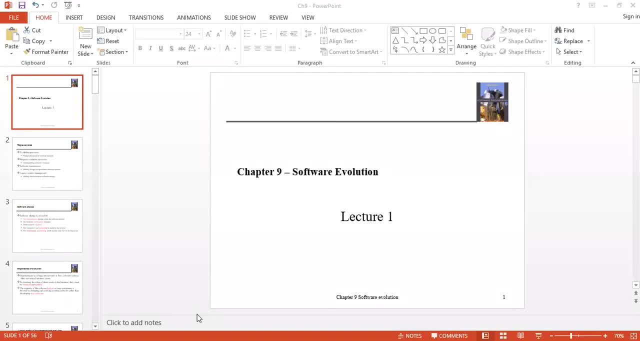 Whatever changes will happen in the software, its modifications will happen. then we have evolution. Where are the other children? Why have they come so late? These are the topics that we will cover today. We will see evolution process, program, evolution dynamics, software maintainance and then legacy system management. 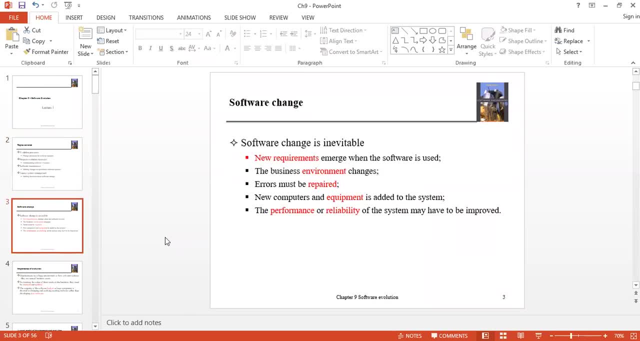 These are the topics that we will cover today. First of all, we will talk about software change. What is software change? Where we add new requirements, Whatever bugs are there in it, Whatever we have If there is any error or fault in it. 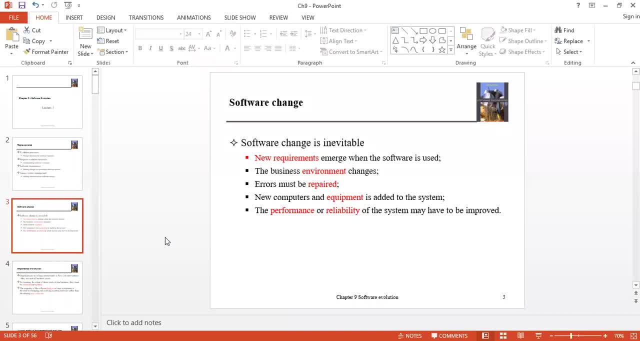 We change it, We repair it, We modify it. Then we have a lot of changes. Where do we use software changes? We use it where we need new requirements, Where we are already using a software, Where our business environment is changing. 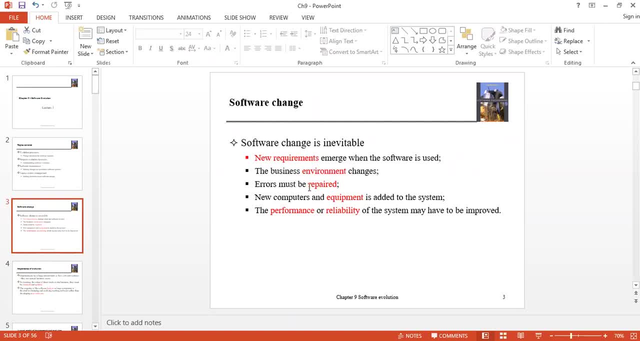 There we need software changes. Error must be repaired. Where we have an error, then we have to do it. New computer and equipment is added to the system. There we need software changes. The performance and reliability of the system may have to be improved. 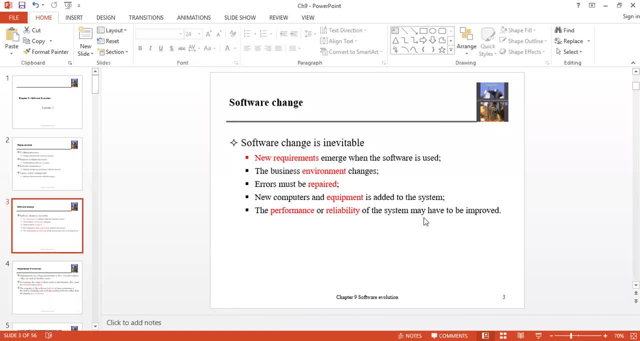 If we want to improve the performance of a system, If we want to improve the reliability of a system, Then we have to modify it, We have to change it. Many of you have already given examples of this, Where we have to increase the performance. 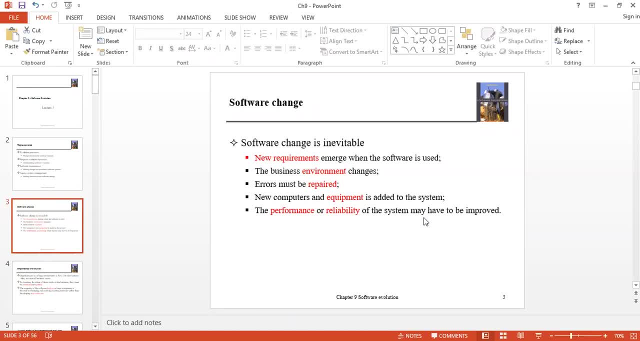 Where is the reliability? If a bug comes in our system, Then how do we change it? Where do we get all that? In software changing or system changing As we want to improve our performance? You have the example of WhatsApp, You have the example of Facebook. 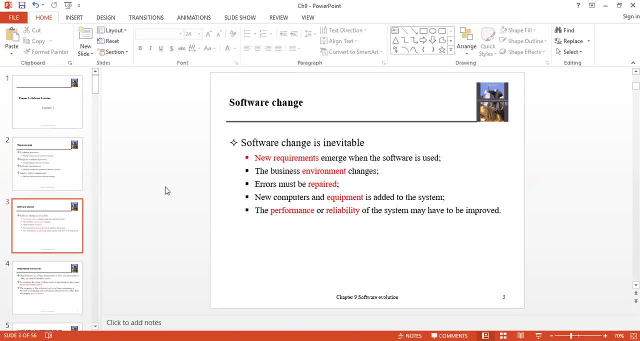 According to your environment, The software we use in our universities. We have those examples. They all lie on it. How do we see our software? You use WhatsApp very commonly. You use Facebook very commonly. We see further in it. We see further modifications in it. There are further additions in it. So all these come in which categories? What are the modifications called? Where are the additions called? What are the modifications called? We will study all types further. Okay, Importance of evolution. What will be the importance of it? 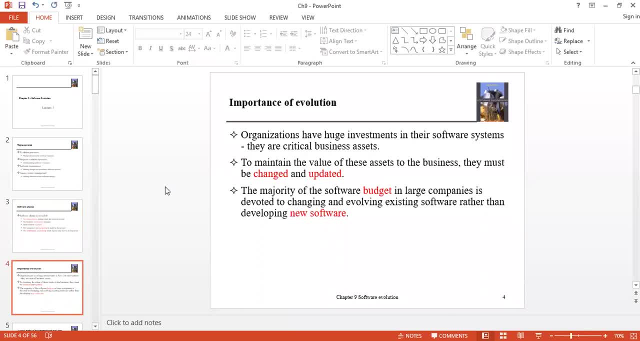 We have the biggest importance of it Where we talk about our business. Okay, So there we have its most important. It is called the organization. How? What we are saying is that organization has a huge investment in their software. The organization invests the most on software system. 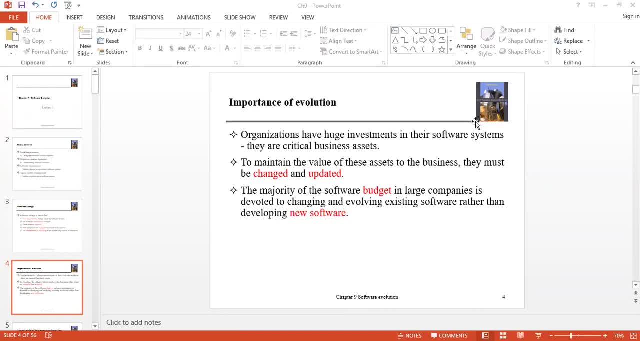 When we look our university's software, LMS is the most common one we have Which is used on a regular basis. Okay, so for our organization, LMS is the most important. It is important for us. We are talking about the important tools. 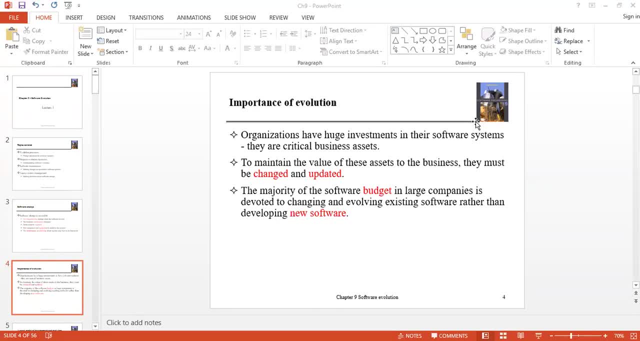 where we have access to it on a regular basis, And the modifications we have in it. whatever changes we have, its usability, functionality, reliability, its easy to use is important to us. So, talking about it, evaluation is important in these places. 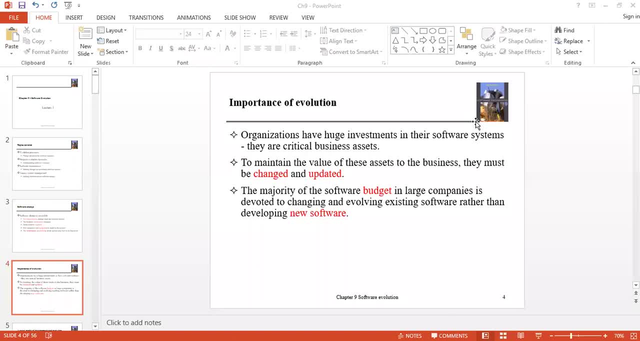 There are many such softwares that are changing with the environment, where we see that if there are two companies and their comparison is going on, if they are increasing their improvement in comparison, it is important for them as an organization To maintain the value of these assets through the business. 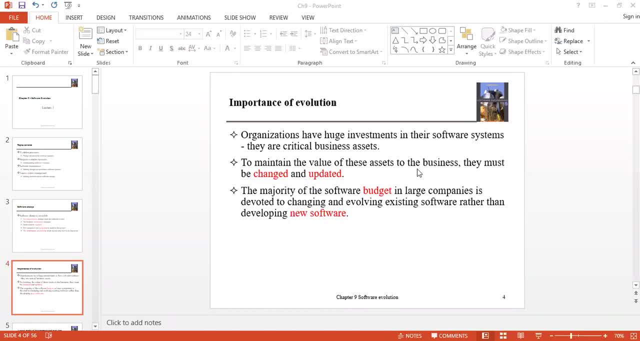 they must be changed and updated. The business example that you gave: the majority of the software budget in large companies is devoted to changing and evolving existing software rather than developing new software. That is to say, the companies that we have. what do they think about their budget? 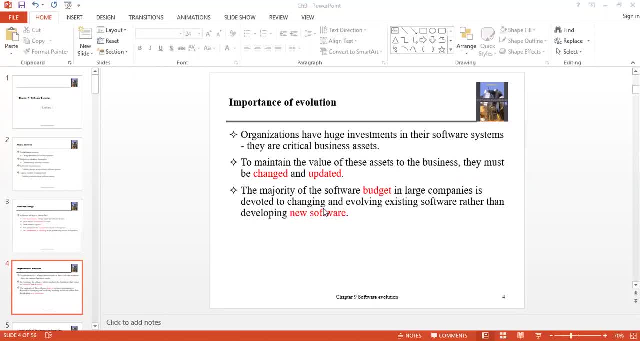 if they develop new software, what is its requirement? If I say it in short, our companies or our organizations, what do they do? The budget on our software, the existing software. they are investing more on its maintenance, they are fulfilling more on its maintenance requirement. 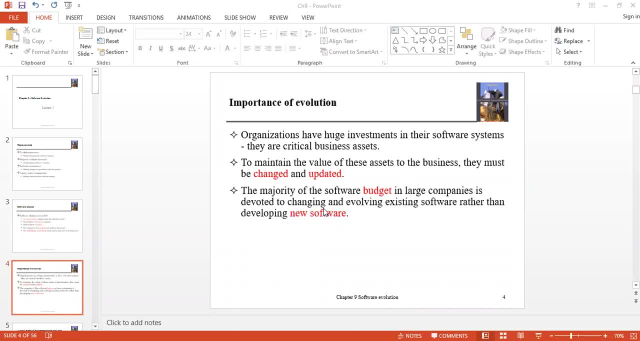 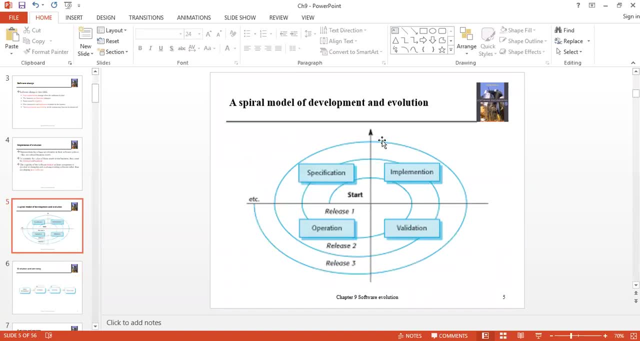 By this we will evolve a completely new software and develop it. Then we move ahead. here we have a spiral model development and its evolution. You all know about spiral. we have it like this: every phase is moving spirally, So we have to reuse it in such a way. 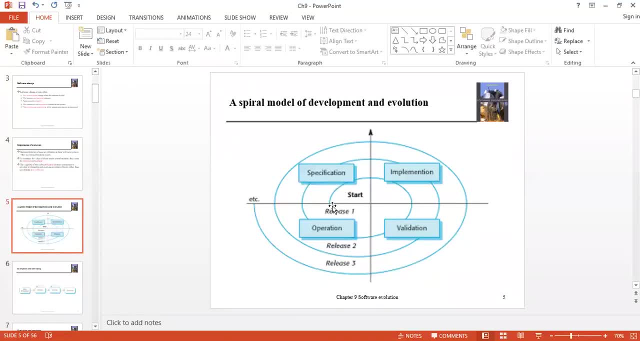 in which all our phases are being covered. We talk about all the parts of it, like the specifications, implementation, validation and operation. So all these parts are moving in this way. so in all this we say it is a spiral In each spiral. 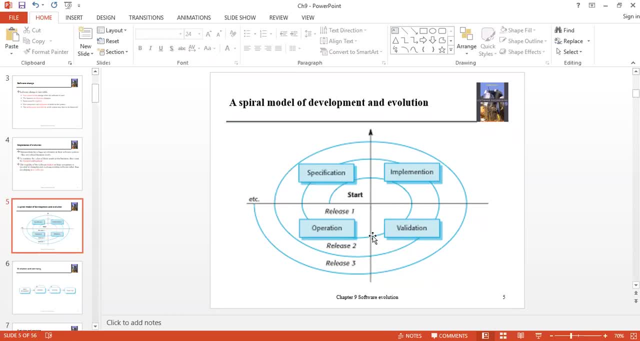 every part is being covered in a little bit. so we have already studied this type in our software process, So its evolution is also happening in this way. So the model is defined. here we go to the next stage, that what is our evolution servicing? 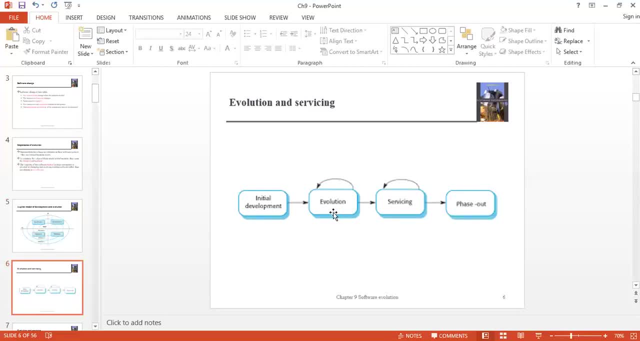 We have an initial development, we have evolution and servicing. What are these two types? We will see in the next slide its definition, what is evolution and what is servicing. And then what we have is that we have a phase out after self-rotation. 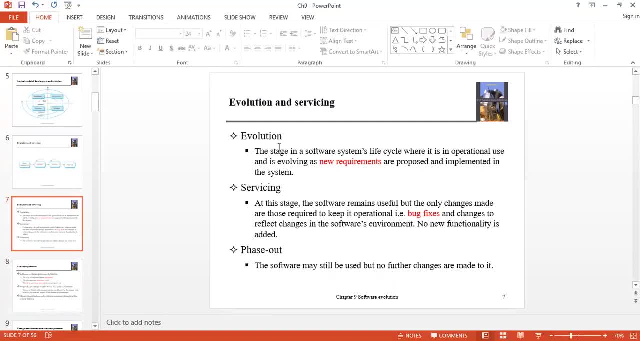 What is evolution servicing? We see that we have evolution, that process where we do in any operation. we have any software system when we add new requirements in it. we call it evolution. What is servicing? We have servicing where we have any error. 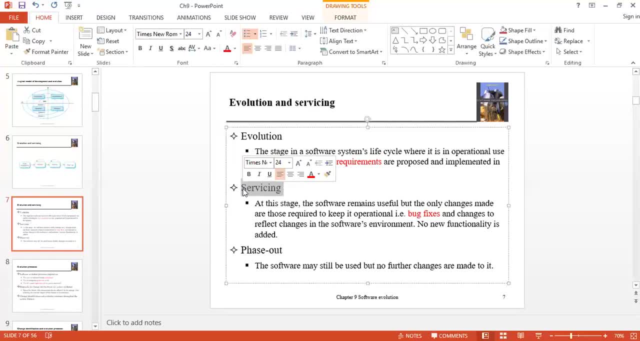 any fault, any bug, to fix it. we call it servicing. Phase out is where we have all the modifications, all the changes that we have to do when we have done the changes. so after that, when we release our system, 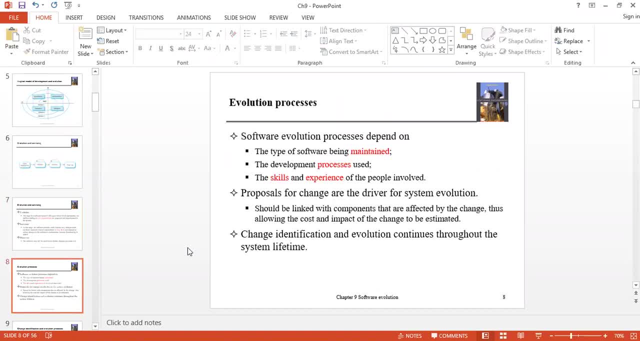 we have phase out, We move to the next move. we have evolution process. What does evolution process depend on? It depends on these three things: on which the type of the software is being maintained, on which it is being maintained- development process- 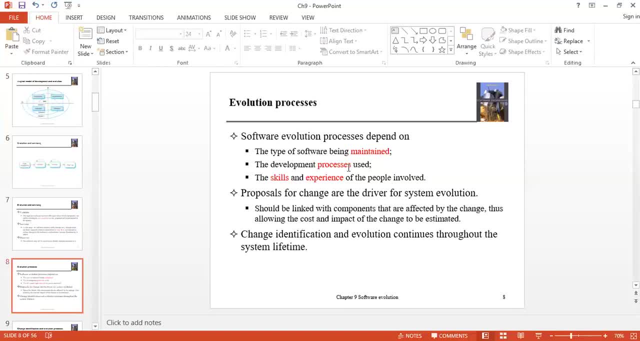 whatever development process we are using: skill and experience, people. These three things we have are such that we have a software system, development process and then what we call those people who have skill and experience. on them we have evolution. it depends on them. 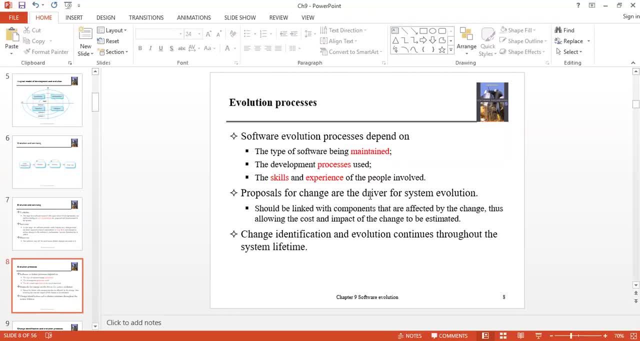 Then we have proposal for change- are the driver for the system evolution. what it is saying is that the components of our system are linked. whatever changes we are having in any system when it is affected, thus allowing the cost and impact of the changes. 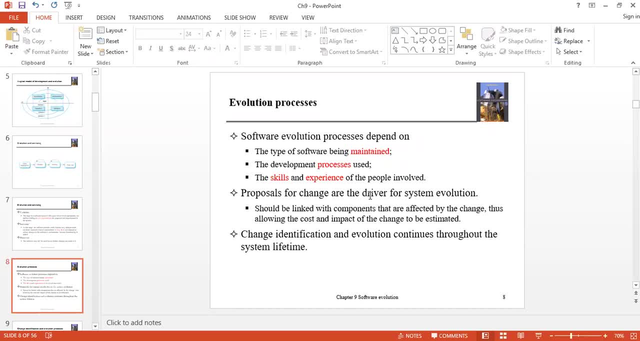 to be estimated, Whatever modifications we are doing in it, whatever changes we are doing in it. so again, on whom it is affecting, on whom it is depending on the cost, The cost that we have on it. it seems like. 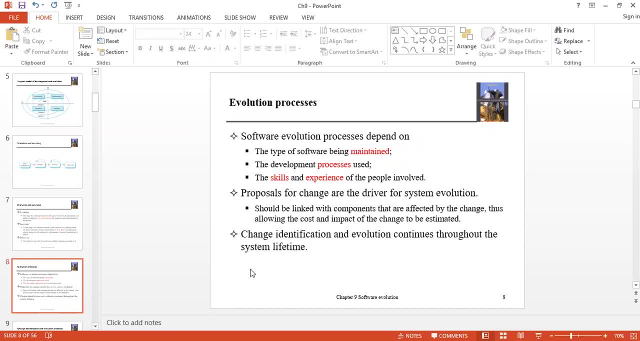 it depends on that. cost, Change, identification and evolution continues throughout the system lifetime. No doubt, whatever changes we are having or evolution is happening, we are implementing it on our software throughout the lifetime. For example, you have Facebook example, you have WhatsApp example. 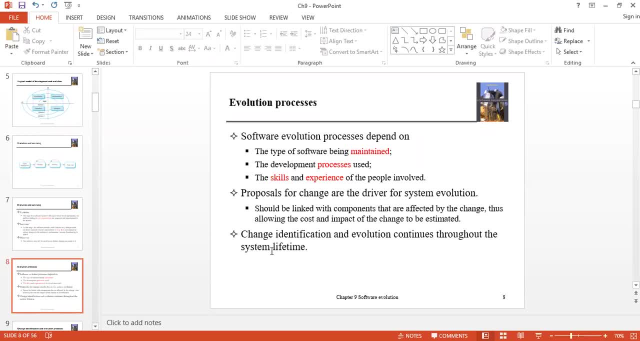 you can see in it that, according to the security purpose, you are changing it in it, that new addition. like you see, if you see one feature, if you are constantly using one feature, and then what happens to you? 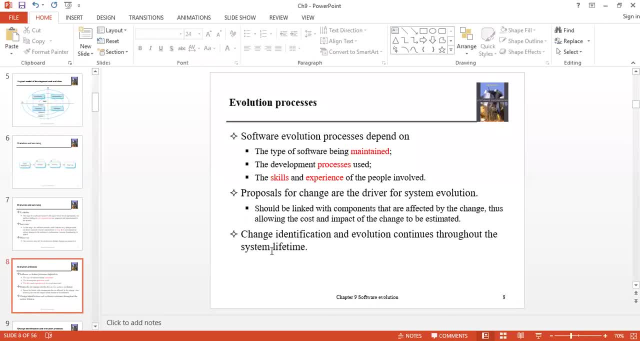 if you start getting bored of it. when its owners, when they come to know that this is our software, these companies, when they come to know that this is our software, by this, our clients, when they start getting bored, what do they do? 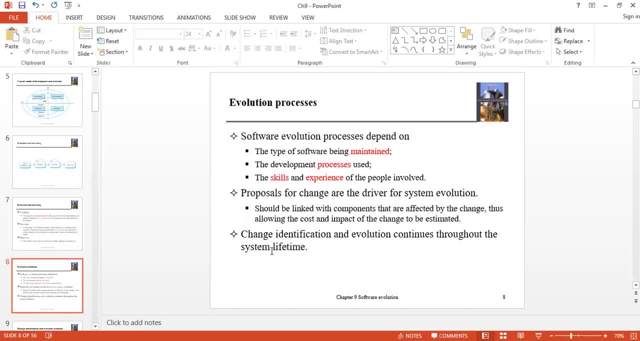 They add something in it. For example, in Facebook, I will see many features like this which are being added more and more. If you see the previous Facebook and the current Facebook, then many features have been added in it. Okay, 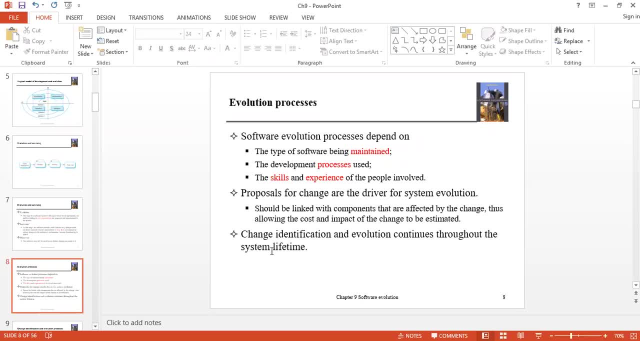 So what we have is: there are important parts, We have evolution, we have modifications in it, we have changes in it, we are talking about adding more parts in it. So what we have is: throughout the lifetime we have. 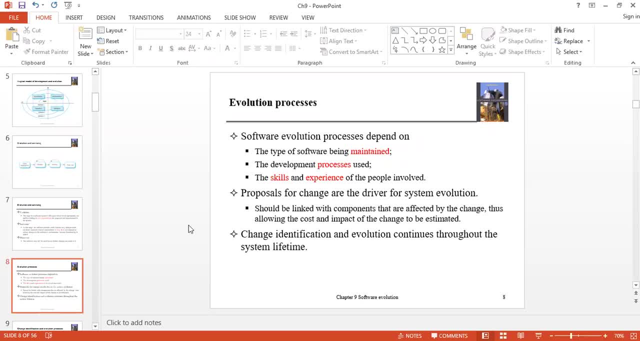 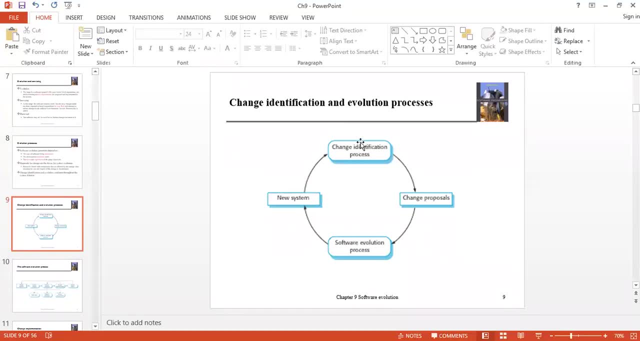 after creating a system, modifications keep happening in it. Okay, So this is what is being talked about. What we have here is change and identification and evolution process. Okay, So what happens is we are talking about what we have. 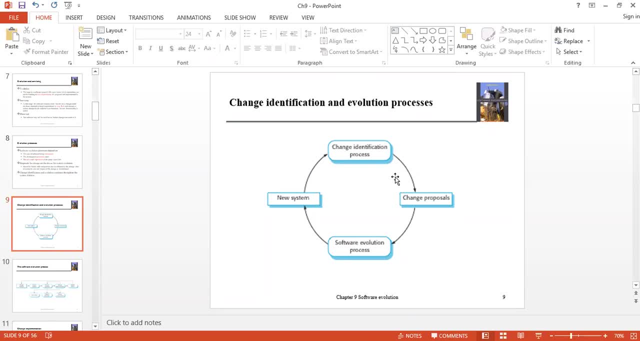 throughout the lifetime, changes are happening. Okay, So we have, let's say it is useful. it is a very important element for us that we are modifying it. So see, now it is rotating. It is in a circular form. 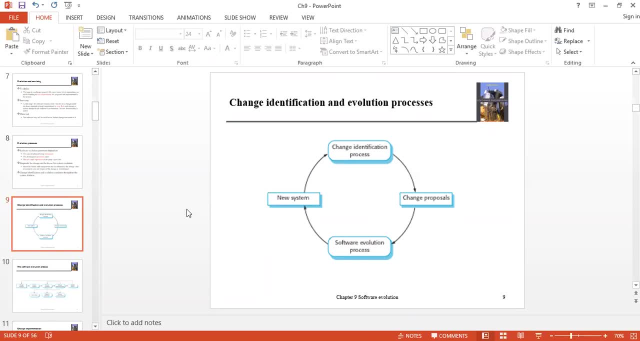 that we are modifying it? Okay, Throughout the lifetime. Then we have a structure: Okay, This software evolution process. We have its process. We have change requirement. What is it going on? Change request: Okay, Change request. where do we get it from? 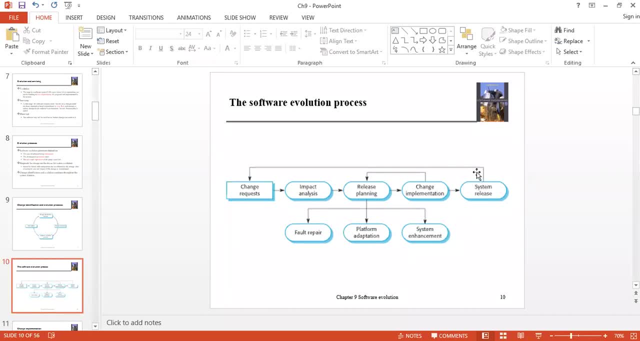 System release. If the system is completely released, if we want to change anything, then we will get its request again. So it will be analyzed. Okay, After analyzing it, we will do its planning. Then, whatever implementation we have in the planning, 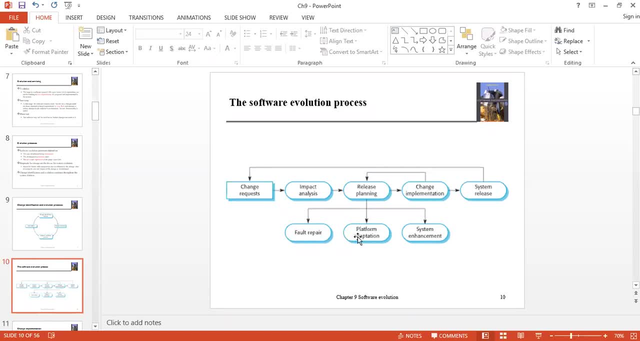 we have these three things. We have to do fault repair, Okay. We have to do platform adaptation, That is, we have to change something in the platform. And then if we have to change something inside the system or we have to enhance something inside it, 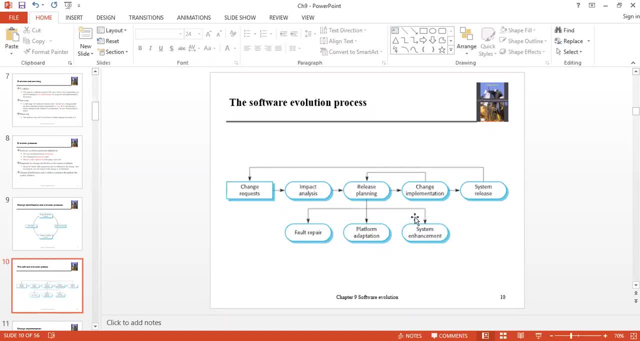 we have to enhance it. So we will get these things in the planning. Okay, We have implementation And then we will get system release. This is one of its steps, Its processes. Okay, We will move ahead. Change implementation. 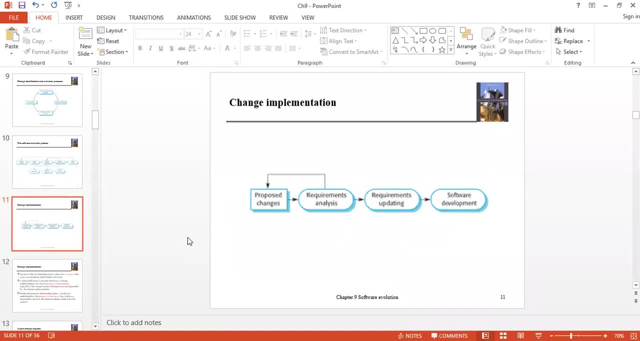 What we have. what we have what we have here, we have proposed the change. Then we did requirement analysis. Then we did requirement updating What we have analyzed. we have updated it. Then we have done software development. 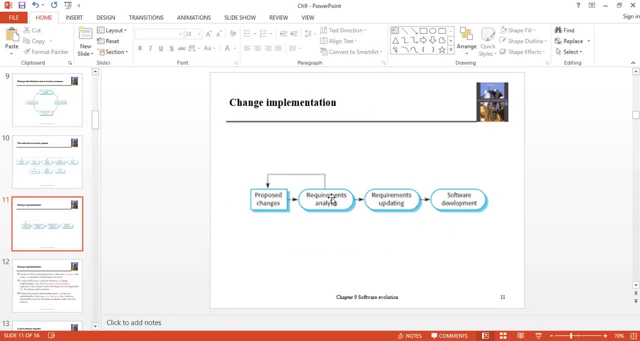 If we have to do any requirement on the initial basis, then what we will do is: from here we will do purpose changes. That is, here we have changed, we have done some system. that is, there is such a model. 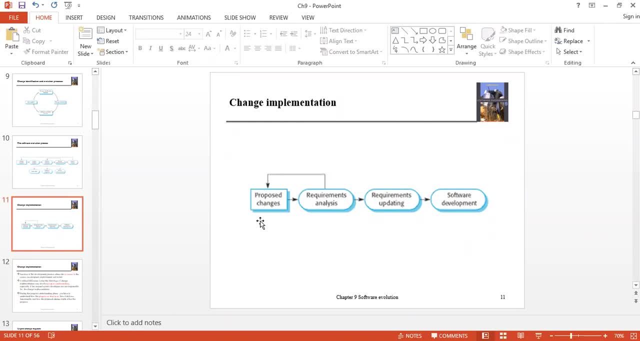 which is saying that after analyzing the requirement, we have come to know that we have to do some modifications in it. So we will move towards purpose changes again. Otherwise, if we are here, if we have finalized it, then move forward. 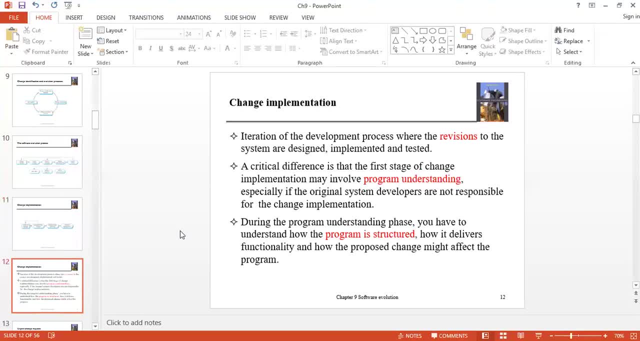 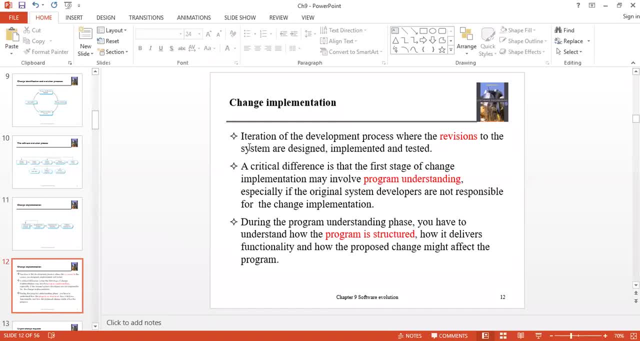 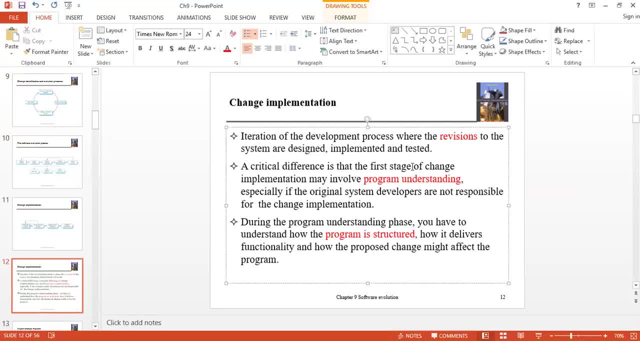 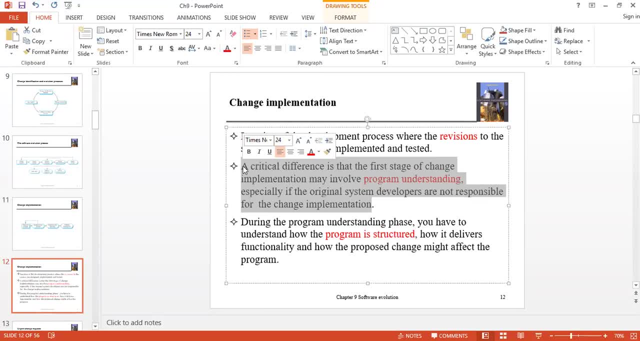 so for him it will be a difficult part, because he will first understand that program, then he will make modifications in it, then he will make changes in it. so this is being talked about here: during the program understanding phase, you have to understand how the program is structured. the same thing is going on, that if you are changing, if the same developer, like I, have developed a program, I have to change in it, I have to make modifications in it. it is easy for me but it will be difficult for you. so what will you do? first you will understand that program part. 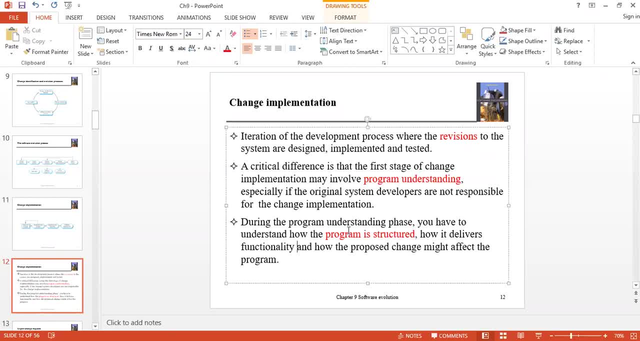 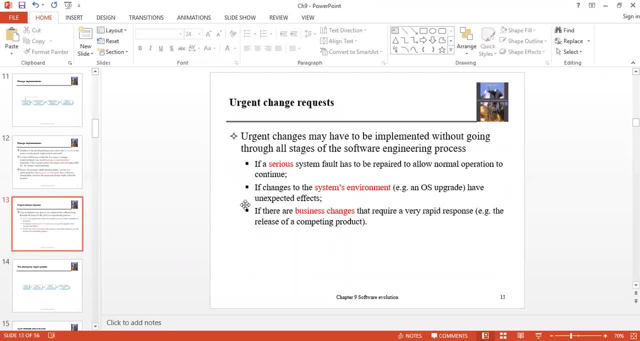 then you will make modifications in it. ok, now this is being talked about here. in the next slide we will move to urgent change request. the urgent change request is the one that we are immediately asked on an urgent basis. For example, I will say to you: you have a system, your operating system is caminho apart. so you will say that on the basis that I want to perform it correctly, because my work is still here and we have an urgent change request, 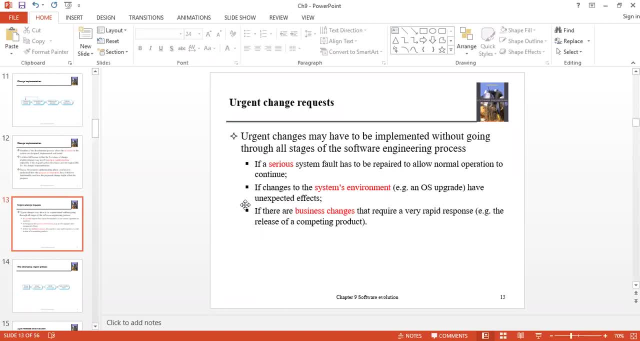 then a hazard is~ Shuka, we have to remove that apple, we have to remove. If there is an operating system problem, you have to remove it on an urgent basis. You have to remove it on the spot. If a serious system fault has to be, that is, if we are working and there is a bug in it. 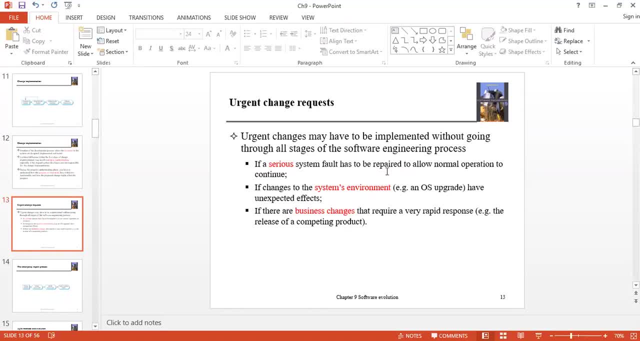 then we have to tell it to a company or a person. For example, if you are solving an assignment, it is urgent for you to solve the assignment At that time. if there is a problem in your system and your assignment is not done, 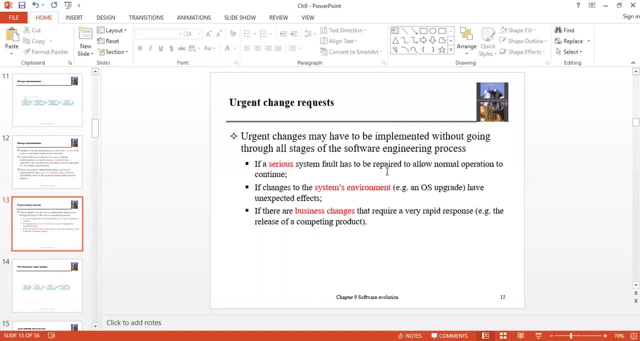 then it is obvious that it is a serious fault of yours. You have to change it urgently In this way. you have to change the environment of your operating system If there are business changes. for example, we have developed the entire software. 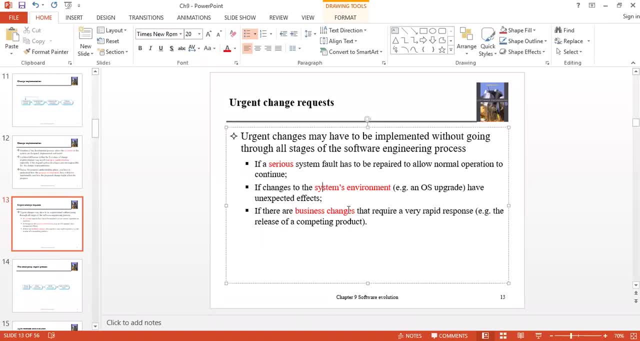 I will give you an example. For example, we have developed an environment system. It was our business change. It was the requirement of our business. We want to add the same thing to LMS and modify it. We have to do online registration this time. 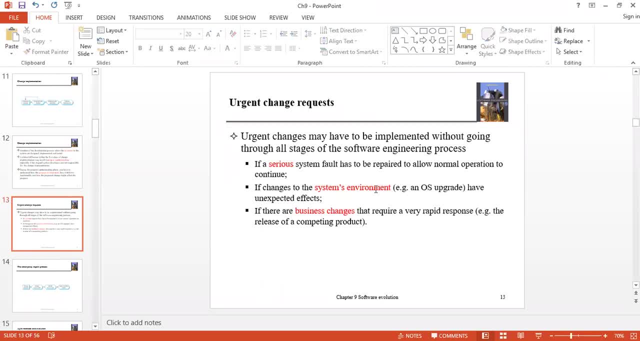 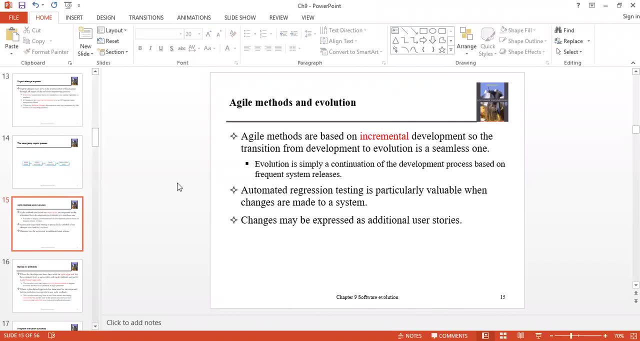 It was our business change. Such things are done on an urgent basis. So it is talking about that Agile method and evolution. You have already read the Agile method. We know this Step by step. we have the incremental form, We have its development sequentially. 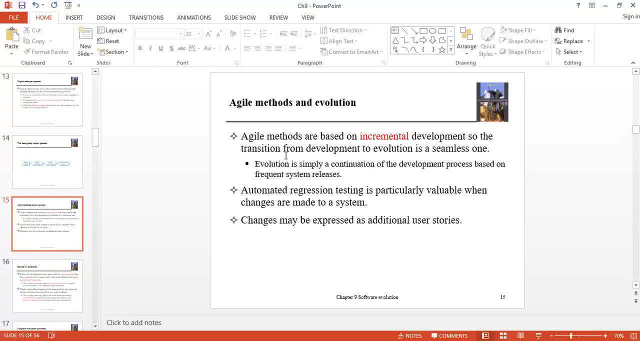 So here it says that we have to do evolution with it. It can be done in one step, It is easy. Evolution is simply a continuation of the development process based on frequent system release. We have a continuation process for any development process. 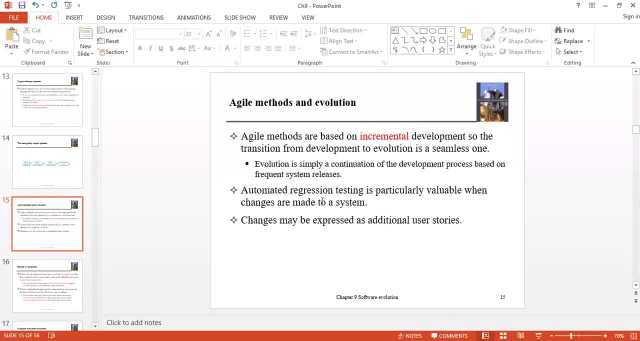 Automated regression testing is particularly valuable because changes are made to a system. That is, whenever we make changes in any system, we should have the testing automated. Whatever modifications we are doing in it, whatever changes we are doing in it, we should test it automatically. 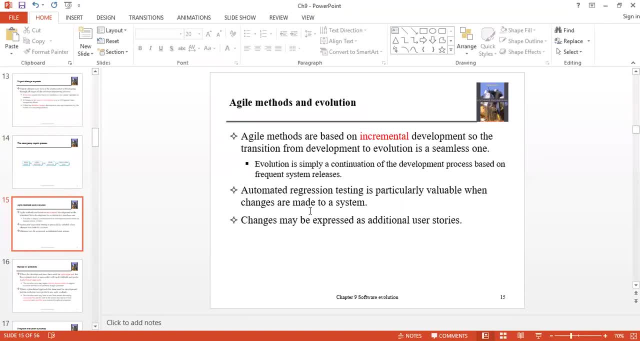 and tell it whether our system is doing it right or not. So we have to do the testing on its backend. We have to do it automatically. Changes may be expected as additional user stories. That is on Agile, when we talked about Agile types. 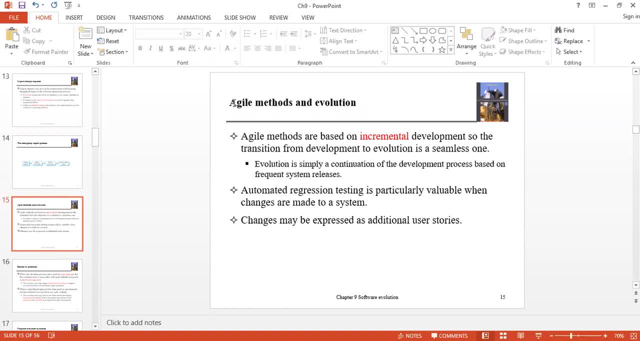 when we were studying Extreme Programming, when we were studying this type, we said that in this, what we do is we do it in Agile method, that we make our users a part of our team. When we make a part of the team, 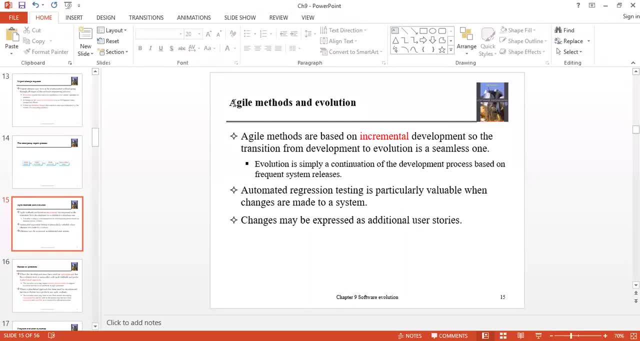 what we do in it is: we collect their stories, We find out their requirements through their stories. So here it says that if we want to do any changes, we take the additional stories of our users and modify their changes in it. Because in our Agile method, 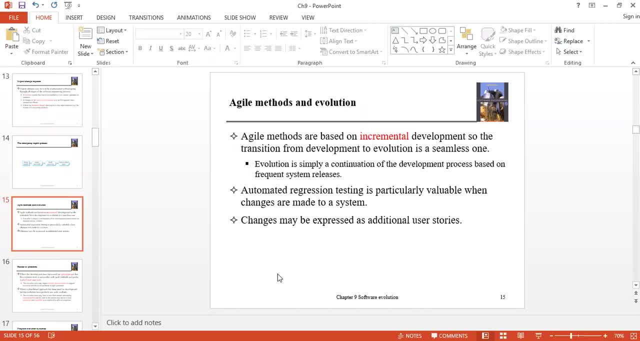 our user is our team member, So we take the stories of our team member, we extract their requirements from their stories and if there is any change we extract it as well. Then it says handover problem. What happens in handover problem in Agile method? 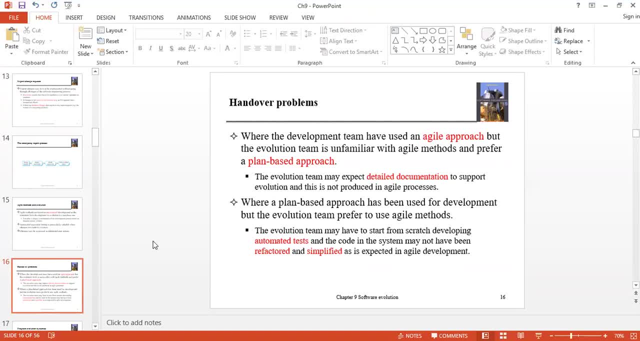 There are two problems in it. If we have a programmer, what he did is the software he developed. he did it in Agile approach. When it comes to maintenance, what happened in the time of maintenance? the maintenance team we had was unfamiliar. 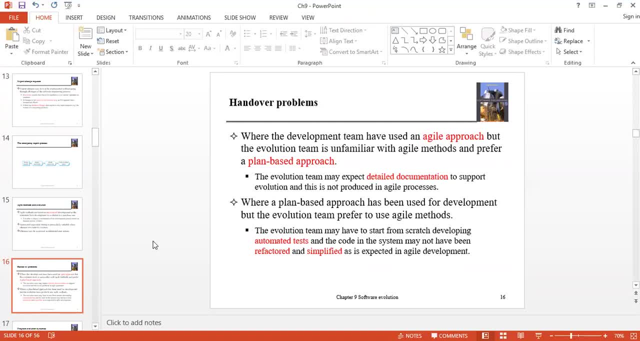 He had no idea about Agile approach. He had no knowledge about it, But he was working on some other approach, For example, there is a plan based example here. Take any other example. He was working on some other plan. He was working on some other approach. 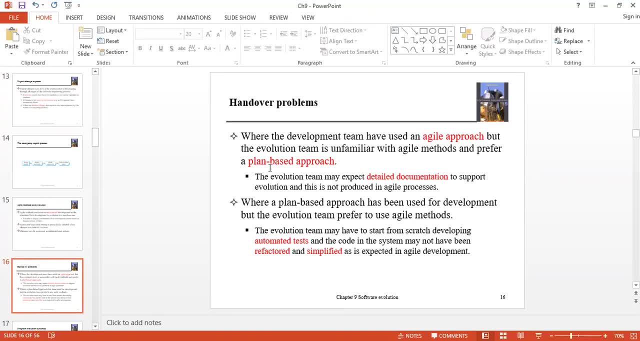 So problems arise here. Okay, Why? Because we have Agile method. What happens is, you know, we are doing its documentation through stories. We are taking its requirements through stories Because in plan based we have complete, detailed documentation. So the maintenance team we have. 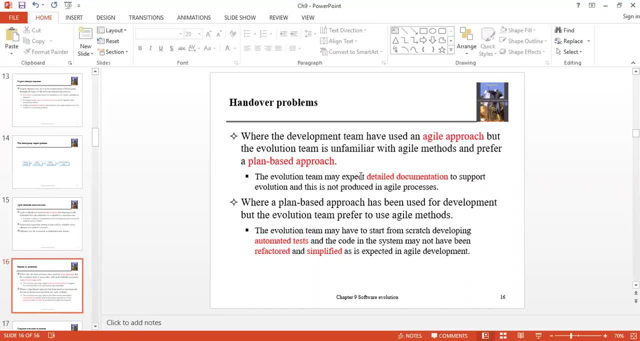 it has the requirement of detailed documentation, Which we don't have in Agile method. So we can do vice versa. Here we have such a team which is familiar with Agile approach. Here we have such a team which is familiar with plan based approach. 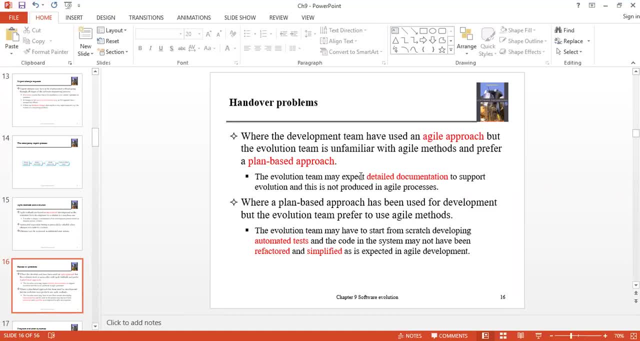 If it is opposite, then obviously we will have a handover problem. Okay, So here in the second point he is talking about the opposite. What is the team we have? It has used plan based approach. The software we have is developed in plan based. 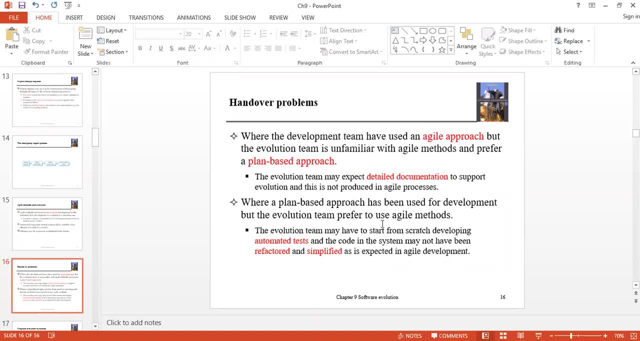 And the evolution team. we have the maintenance team we have, which is familiar with Agile method. Okay, What is the difference in this? If we have used plan based approach, then in plan based, the evolution team may have to start from the scratch development automatic test. 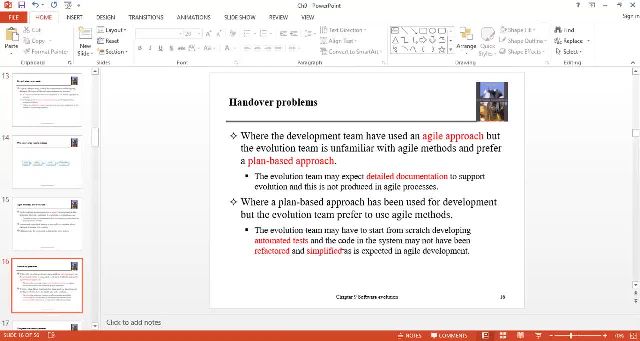 Okay In that they start the automatic test And the code in the system may not have been refactored and simplified. That is in plan based. we have such a system which is not easily refactored, as it is expected in Agile method. 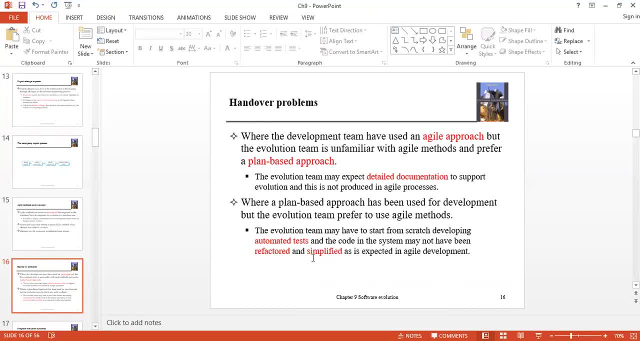 That is, it is not so simplified as it is in Agile method. So what happens is a little light comes on it and a little problem arises on it. Okay, We move to the next point: program evolution dynamics. What is the dynamics we have? 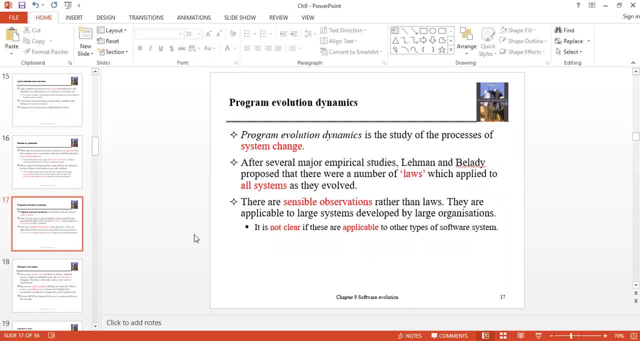 You know that we can call it a movable thing, Okay. So when we talk about evolution, what will come in it? Constantly? or we have a process in which our system is changing continuously. It is changing dynamically, Okay. So what is this? 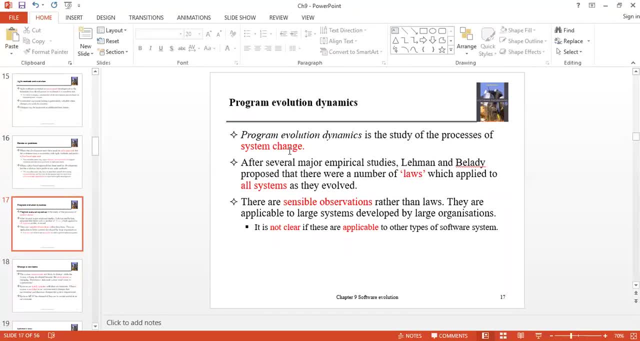 So what is this Program? evolution dynamics is a study of the process of the, that is, a study of the process of system change, That is, it talks about the changing of the system. Okay, We have to refer to the changing. 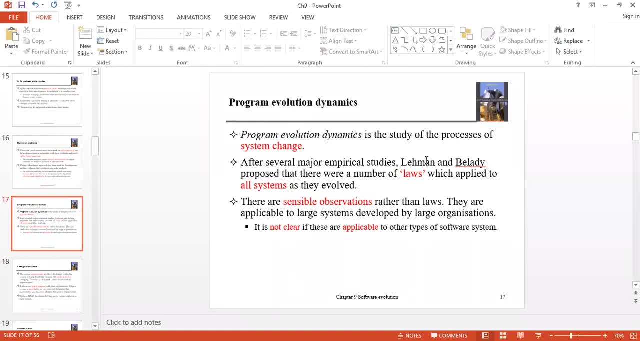 of the evolution After several major empirical studies. here we have two, that is, Lehman and Bellady. Okay, What did these two do? We have some laws that have been referred to us that we have some laws that are applied. 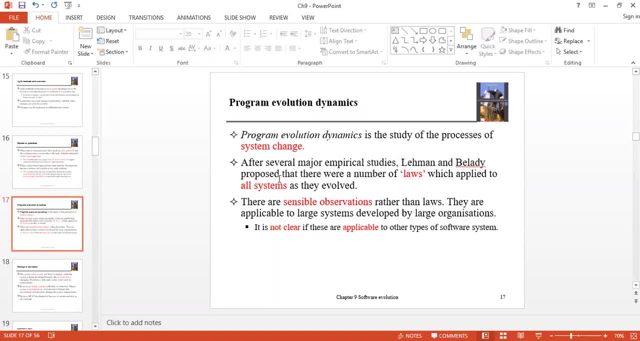 Maximum, call them, or all systems, call them, which we use for evolution? Okay, For its evolution, we have. they have referred some laws that we have defined. Okay, So we will come forward and read Lehman's from this: Okay. 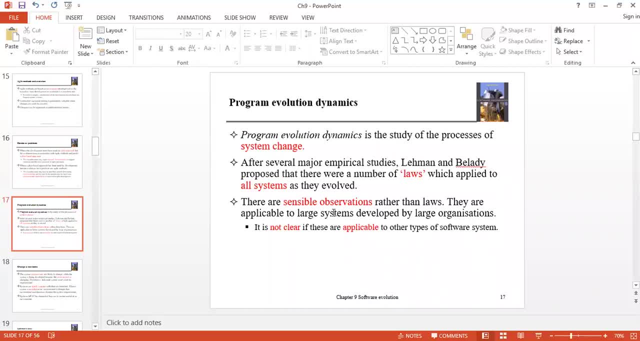 There are sensible observations. This is being talked about here at the third point. There are some sensible observations here as well, which, rather than laws which are being applied to us on a lot of software, on a lot of companies, 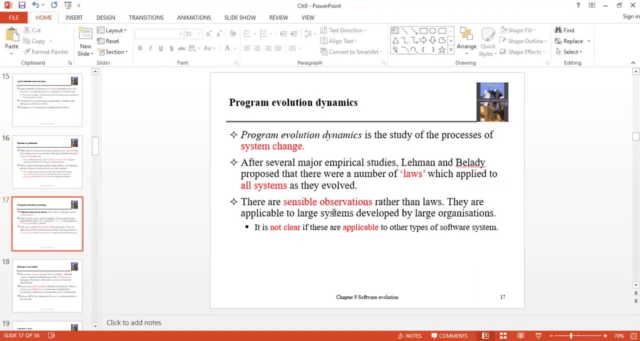 Okay, We don't just have laws that they have defined, we have some observations as well. Okay, It is not clear if these are applicable to other types of the software system. That is, they are saying that we have laws that we have defined. 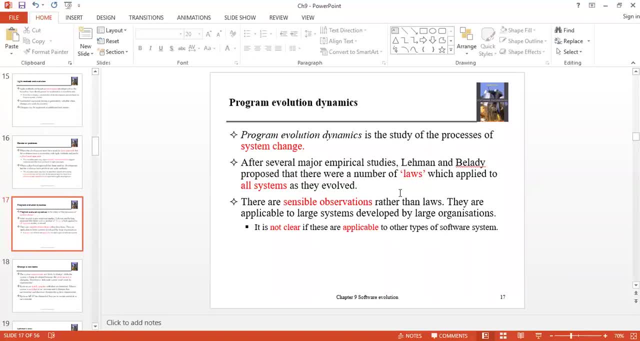 that we have laws or sensible observations. Here we have sensible observations. It is not clear to us that we have applicable or are being applied to other types of the software system. Okay, Who are they talking about? On which are they being applied? 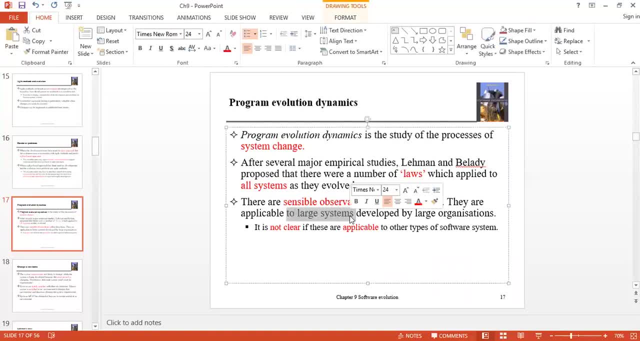 Sensible. we have. it is being applied on a large system for large companies, Okay, Or large organizations. So they are saying that we don't have. it is not clear whether it is being applied on small or medium size or not. 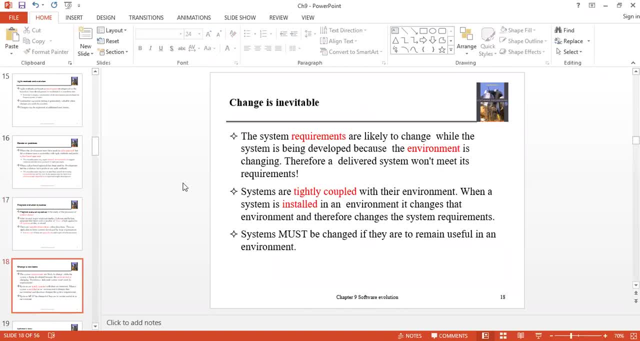 which we have These types? Okay, Changing is inevitable. Okay, What does it say? The system requirements are likely to change while the system is being developed. What do we have? The system requirements are being changed. Okay, During which. 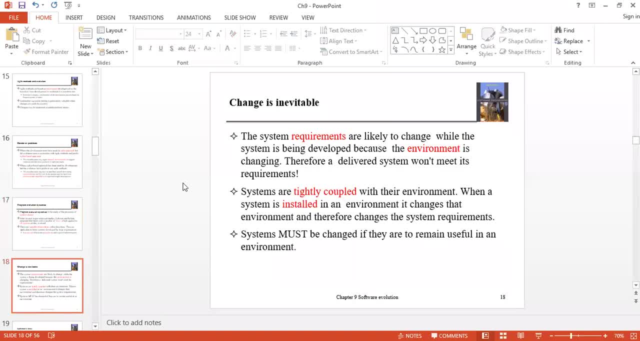 During the development of the system. Because the environment is changing, therefore, our delivery system won't meet its requirement. It means that our environment is changing from time to time, So according to that, our requirements are also changing When we deliver. 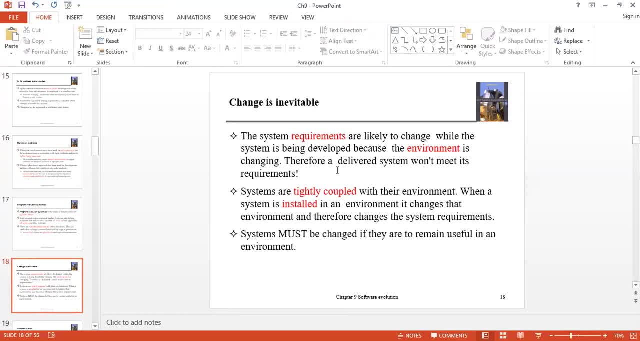 our system. what happens? Our personal requirements are not being fulfilled. Its requirements are not being met. Okay, Systems are tightly coupled with the environment. That means the system we are making is coupled with the environment As soon as we install our system. 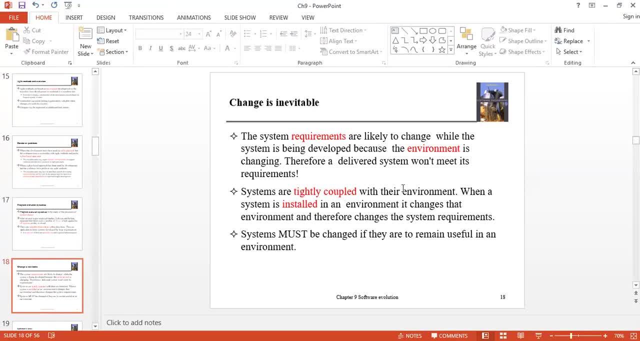 with our environment, some changes occur in it. Okay, So we have affected the requirements of our system due to those changes. Okay, Systems must be changed if they are to remain useful in an environment. Okay, It is said that our system 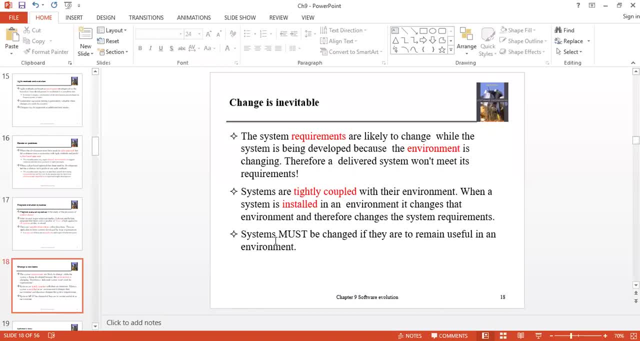 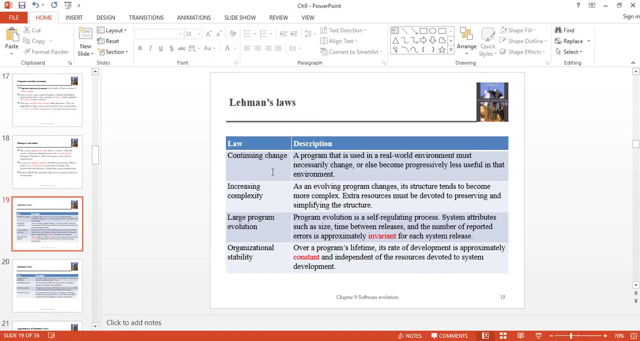 must be changed. It is mandatory that it is changed if it is useful for our environment. Okay, We will see how we must change it in seven laws. Okay, We have a law in which it says that continuing change in its name is a law. 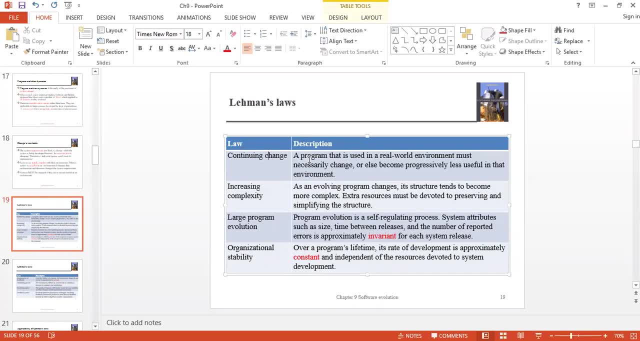 You can guess from its name that the system must keep changing along with the environment. Okay, Whatever real world environment we have. Okay, In increasing complexity. it is saying that as we keep changing in it, the system will be more complex. Its complexity. 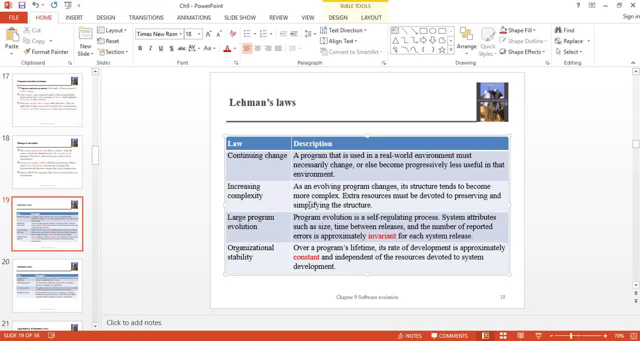 will increase. Okay, It is saying to reduce it, but what we have to do is that we have to add such resources to simplify the complex structure. Okay, In large program evolution, it is saying that program evolution is a self-regulating process. 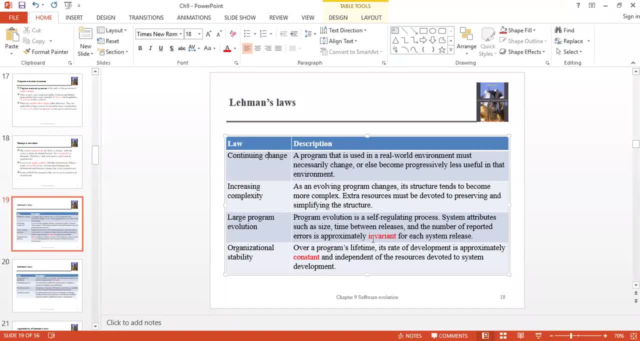 System attributes, such as size, time between release, any number of reported errors. evolution is invariant, ie its size, its time, its error. If a large program has one system, then there is something else for it. If we have small, medium, whatever evolution of the program we have, we have these changes. we have these things. 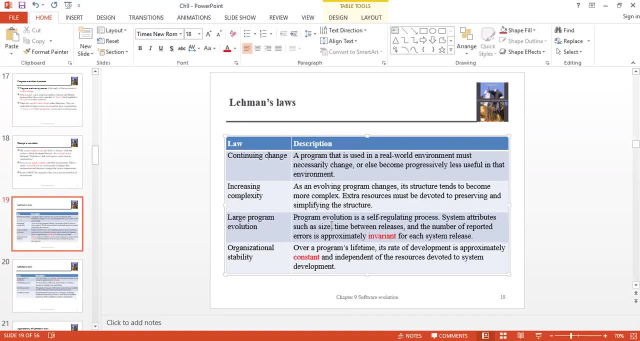 It depends on each software system, It will be invariant. Organizational stability: What does organizational stability mean? Over a program's lifetime, its rate of development is approximately constant. For organizational stability, the development we have is approximately constant and independent of the resources devoted to the system development. 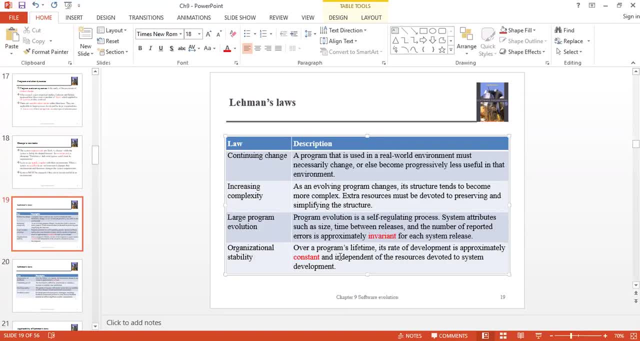 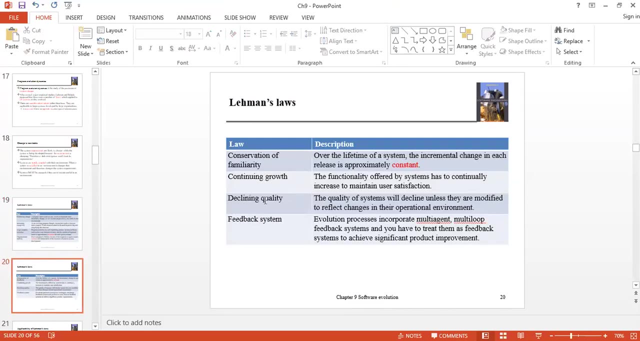 ie the development rate of the program should be constant. This is defined by its law. Next, let's move to the conservation of families. Here we have the conservation of familiarity, which means continuous growth and declining quality and feedback system. 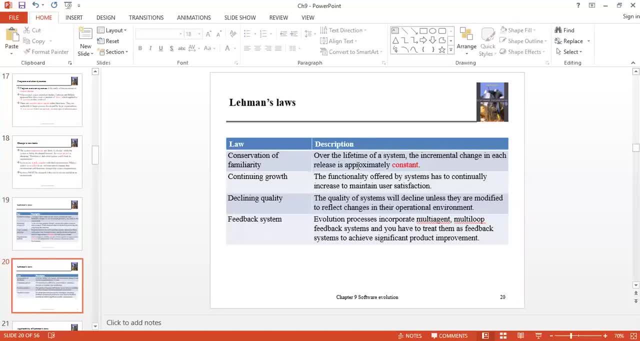 What does it mean by conservation of familiarity? It says that over the lifetime of a system, the incremental change in each release is approximately constant, ie whatever we change in each release should be constant. This is the law of its description. What is this continuing growth? 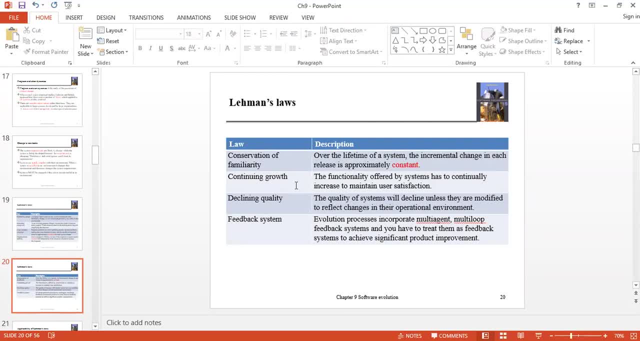 It is obvious from its name that whatever software system we have or whatever system functionality we have, system the functionality here was, may I'm constantly gonna tell you, spoke in. please wanna tell you it's the under job. you have our a casket. thank you, it was honey. died at the users key satisfaction hotel at the gate. yes, I'm. 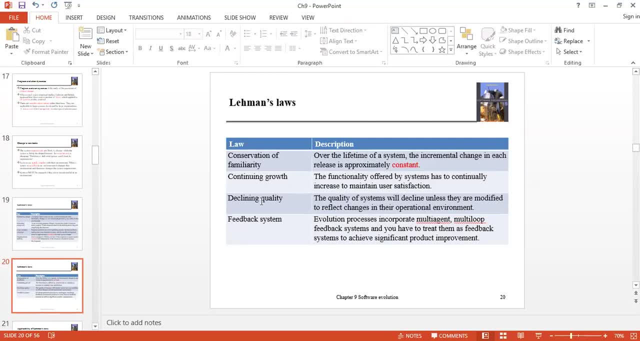 a log of the ECM of a bar step of Facebook. while example easily apply, holiday care, declining quality. the quality of system will decline unless they are modified to reflect in the in the operational environment. are you about each? are you a quality decline? come on, we can look at the under the. 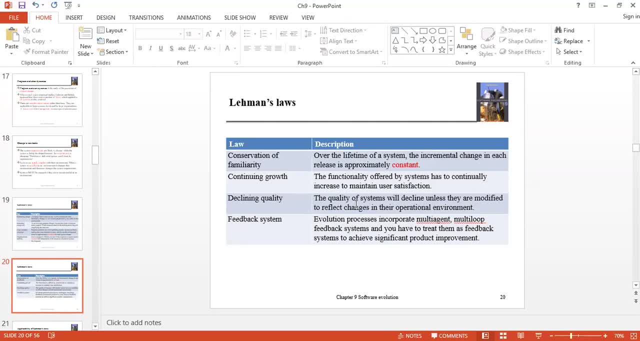 hand modifications. cartage, are you your modifications? are you a reflect, a receipt? any more ticket to my bus? quality decline. feedback system of local question names in the authority. feedback: I'm lady and take care from the users, Kelly, from the client. a little bit feedback I'm accept. 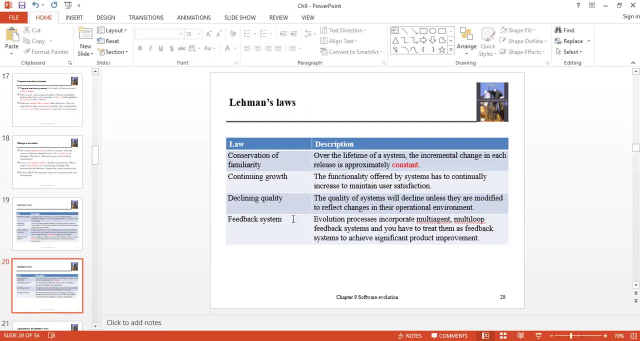 carrying gay the work yoga. I'm not as a positive language for the improvement killers could use that in me. okay, you gonna make some of the software job look publicly used, cutting up a place, trusted leader or download circuit or something. they focus you in the box a. 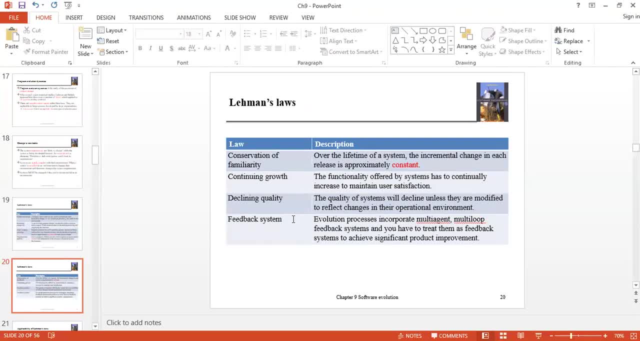 feedback monkey, so sweet, back a massive. you attack a problem on, say, well, I've got feedback. here is a couple of us to use. turning across the feedback. there are those kind of those modification. can you host a stop, say, modifications cutting it was improvement, but I didn't him. yeah, they. 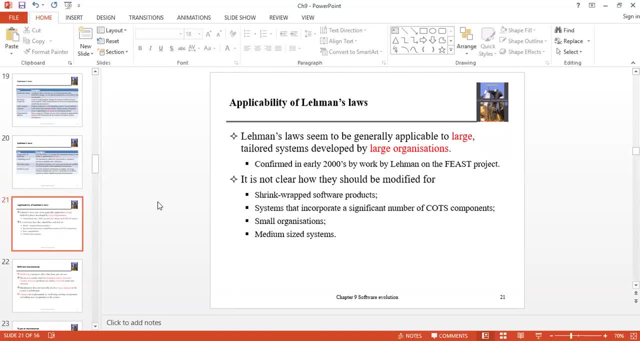 have my bus again. I'm alone. I'm alone, okay, I read. seems to be generally a character applicable to large tolerated system dealer by life of me, and they get to it. so much though my bus Joe, my policy limits lawyer, yeah, how happy apply. or a large systems pick joke a dealer, because I think it's. 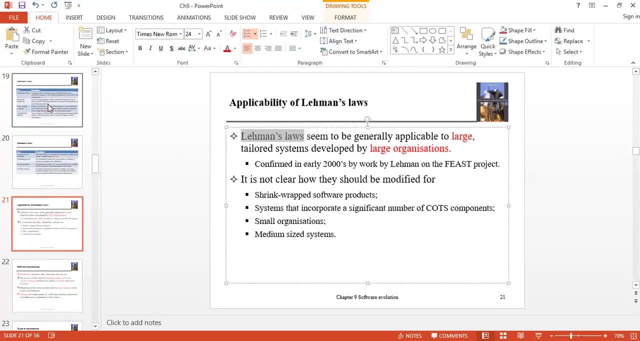 terrible by large organizations. yeah, it's kidding me, I'm a gets- are a loss for an AI. so yet the Hopkin companies are practical and he can come. why in early 2002 by work bile miss on the fish project, take a project to come together. 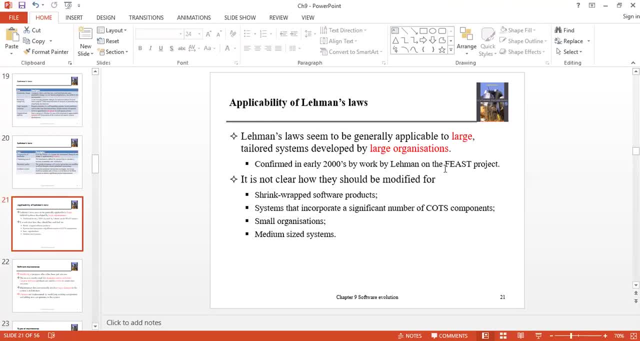 though it's too person, I play a sorry loss. the director, it's a maha pick, some from Canada. it is not clear how they should be modified for any character is. he has applied for large system where it is not clear where it can be modified. shrink and wrap softwares products means small shrink system. 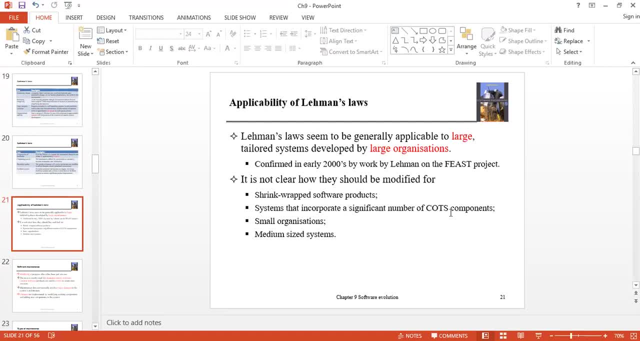 system that incorporate a significant number of force components. small organization or medium size organization means he is talking about it is applicable only for large, but he has not applied on these types of softwares. he has not applied on these types of softwares, whether it is beneficial or not. 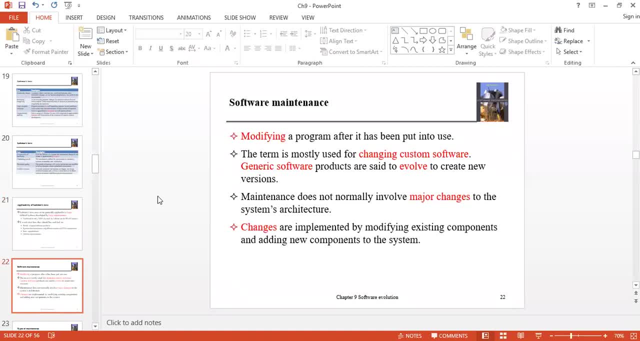 software maintenance. we have modification of a program after we have taken it in use. what is maintenance? we have a program, we have started using it. then we have seen this box in it. we need this changing, so we call it modification, we call it maintenance. the term is mostly used for changing custom softwares. 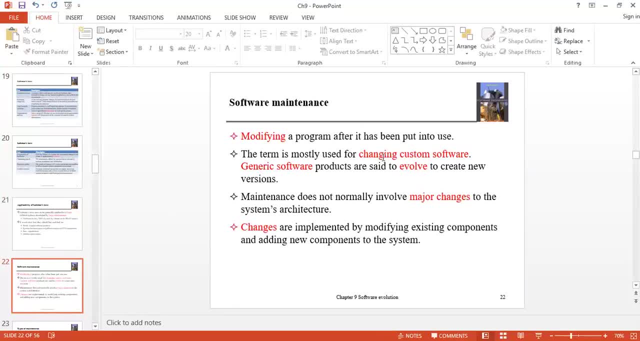 we use this term for maintenance for custom softwares, but for general softwares we use word of evolution. we create new versions for this. we use word of evolve. for changing, we use word of custom softwares. ok, maintenance is not normally involved major changing meaning. when we talk about maintenance, we dont talk about major changes. 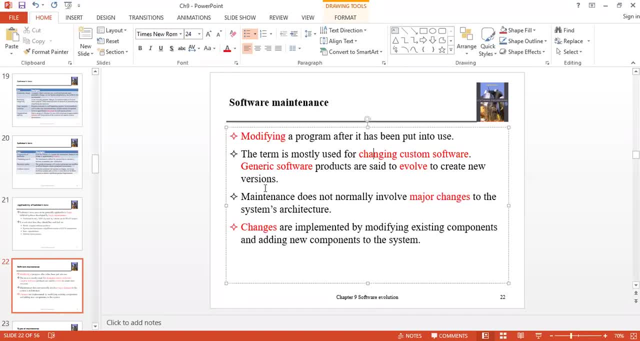 but small changes, ok, to this system. changes are implemented by modifying existing components. we are talking about something: existing component, adding new components to this system, meaning in it is addition of new system and we are talking at small level, that we are changing types of maintenance we have here. 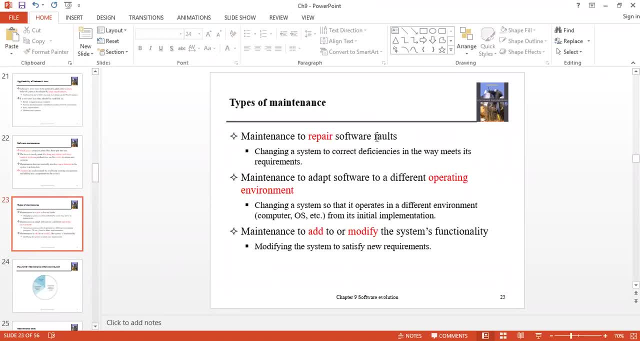 maintenance. maintenance to repair software fault, that is we are repairing any software fault. then maintenance to adapt software to a different operating environment, that is, we are changing its operating system. then maintenance, that is some add or modification. we have these three types. we are repairing any fault in any software. 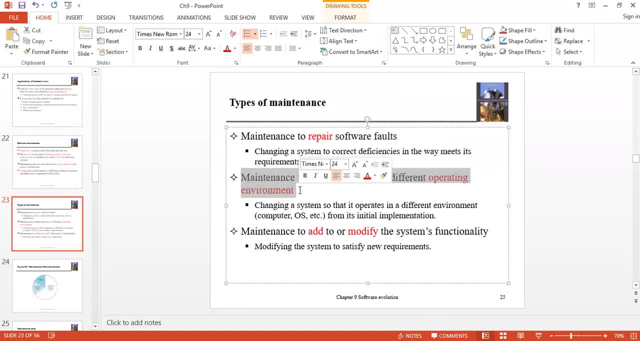 then we are changing any operating system, then we are adjusting our software according to that and we are maintaining according to that add or modify this system functionality. we are doing some addition or modification. so these are the three types of maintenance. we can see the ratio of these types. 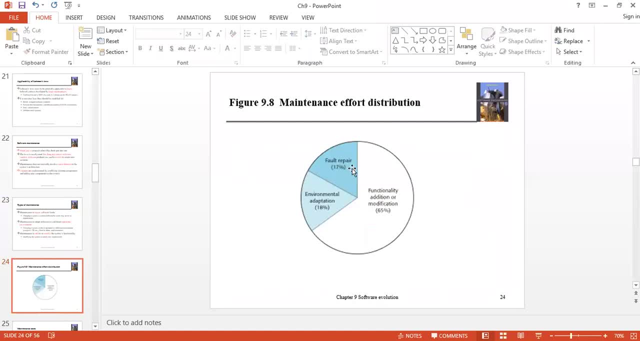 through this pie graph that what we have fault repair, we have 17%. if we look at environment, we have second type here. second type is this one. so in this, how many percent it is 18% remaining? we have functionality, addition and modification. how many percent we have 65%. 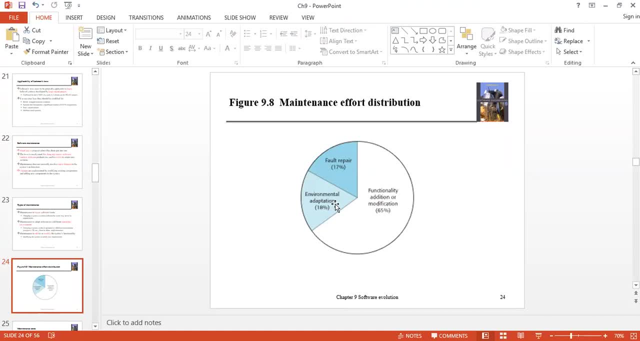 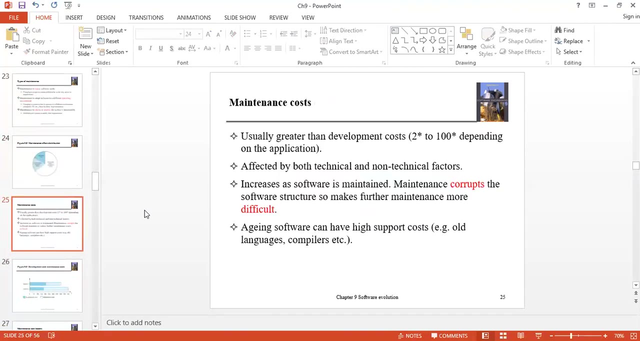 so this is the distribution graph, how it is distributed. we have three types that we are doing three work in any system in its maintenance. so how we can define these three types. so this is the distribution graph. we are talking about maintenance cost, what is mentioned in this usually. 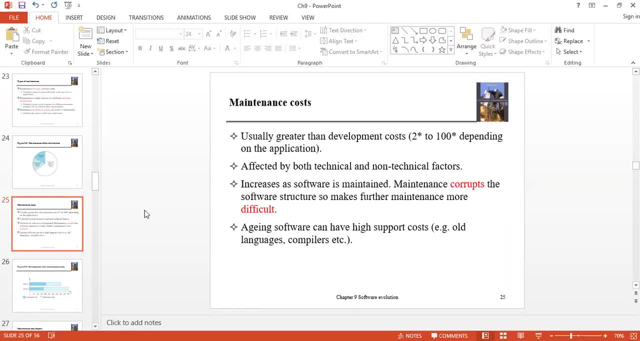 greater than development cost means that the maintenance cost. we will see in next slide how much difference we have in development cost and in maintenance cost. so what we have, maintenance cost is always more how you can take an example of this. so how many software essence we have done earlier. 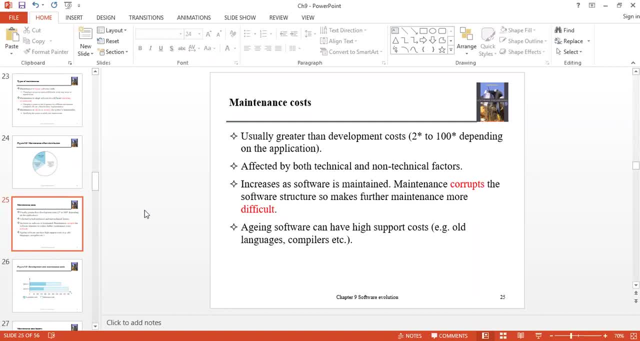 we have developed like, if you see facebook, i remember when i entered university in 2010-2011. since then, our facebook has come when i used it for the first time. so till now it has developed once. and then what is happening in it? only modifications are happening. 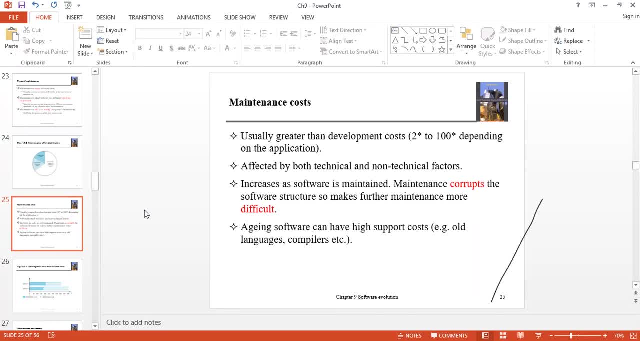 so what is that? the post of its development only took one day after that. what is happening in it? till now, we have maintenance cost applied in it. so it is said that we have maintenance cost which is usually greater than development cost effect, by both technical and non-technical factors. 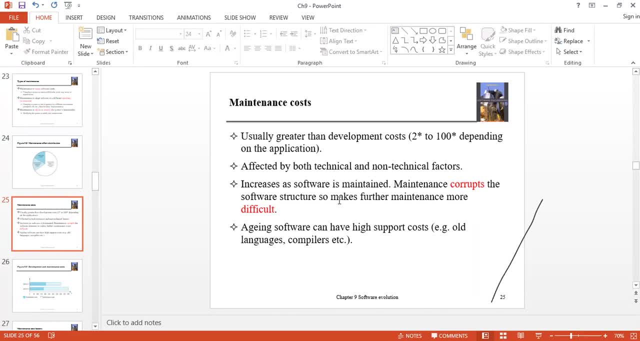 in case as software is maintained. maintenance of the software structure, so make further maintenance more difficult, means what is being said: if we apply one maintenance, then that software structure will be affected a little bit. so, along with that, what we do is we add more maintenance in it. 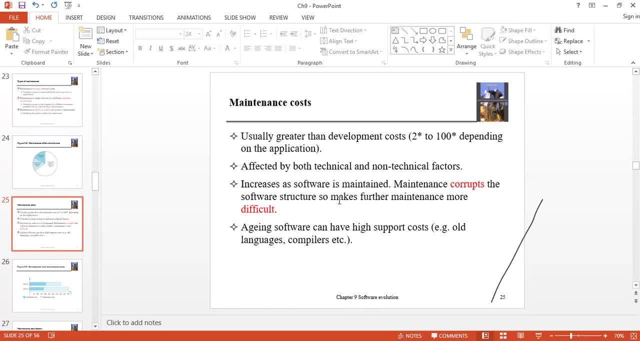 so what happens to us? we have a little bit difficult process because we have sometimes it happens when we are maintaining, then we have other components or other things which we have its parts. they are affected. ok, so on that, further modification, further maintenance is required. aging software can have high 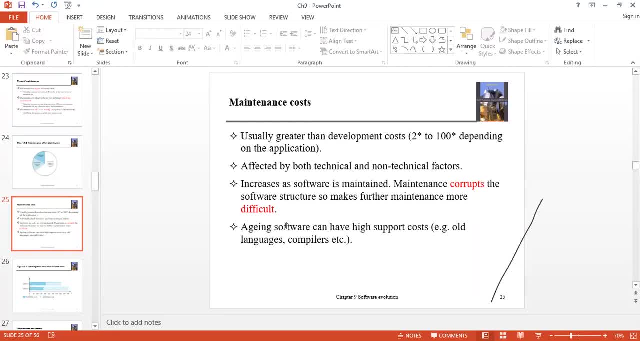 support cost means- this is what is being said, as i just said, that the pranic software son what is being said- that we have pranic software. its cost is more. for example, now we are new, we are new software developers, pranic languages used, pranic compilers used, 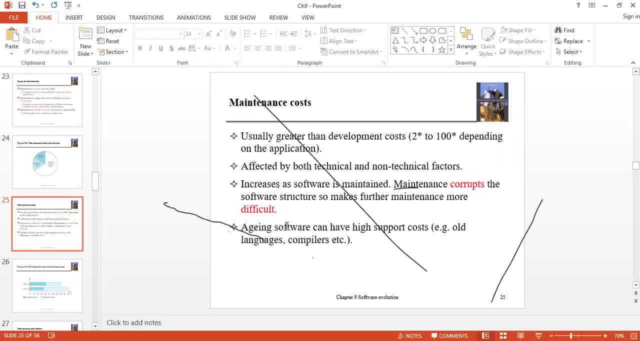 it again. who is saying this? i will mark everyone absent. is this clear? everyone was absent in class. why, ma'am, why are you marking everyone absent? who is doing such a thing among you? no one came from outside, ma'am. what are you talking about? these lines coming up? 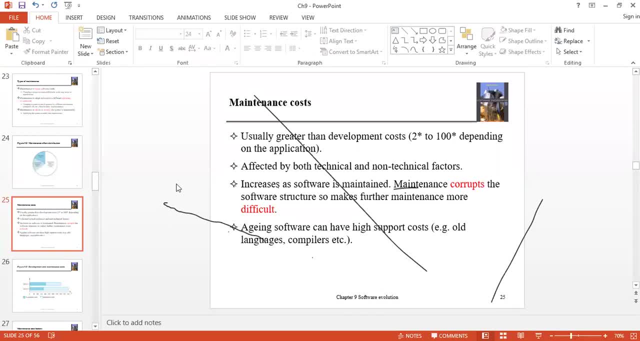 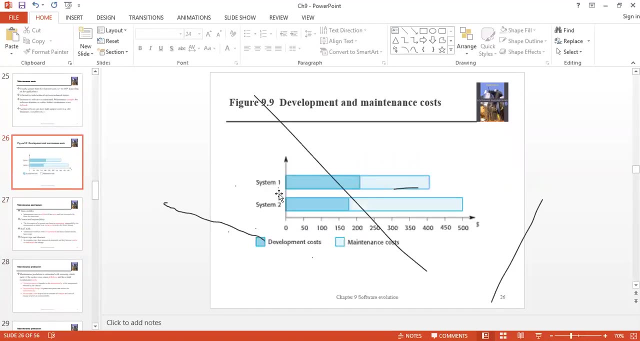 ok, these lines, one more line till. here it is clear. ok, then we move next. this is our slide, in which we are telling that we have this size of a system and second, we have this size of a system. ok, we have large system and small system. so in that, 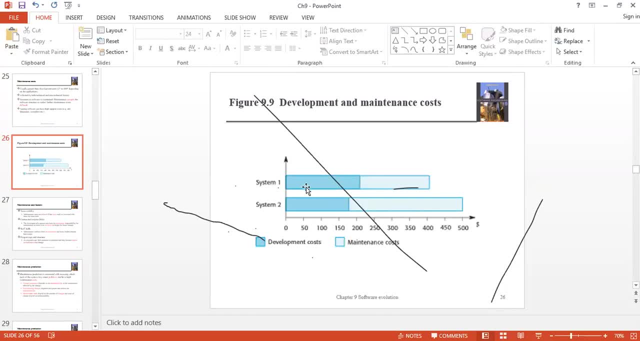 they are telling that see from where it is affecting development cost. we have this and after that we have maintenance cost. ok, so as we have large system, so in that we have this system, we have developed it, so after that we have maintenance cost in it as much as we have. 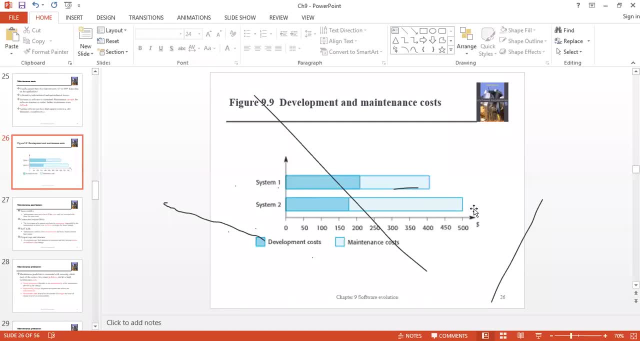 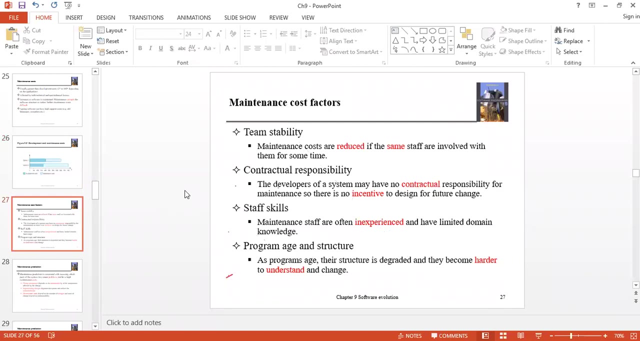 maintenance. it will increase after that. what is happening in it? it is increasing. if it will require more maintenance, then more what will happen? its cost will increase. this is being said here. ok, next we will talk about maintenance cost factors. ok, which maintenance cost factors we are depending on? 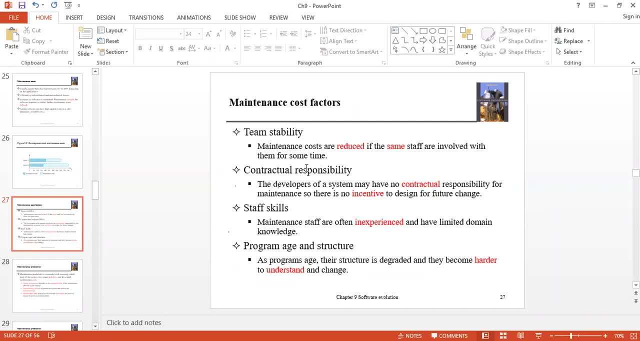 we are depending on stability, ok. we are depending on contractual responsibility. we are depending on staff skill. we are depending on program, age and structure. these four things we are depending on, ok, what we are talking about: team stability. maintenance cost will be reduced if we have the team. 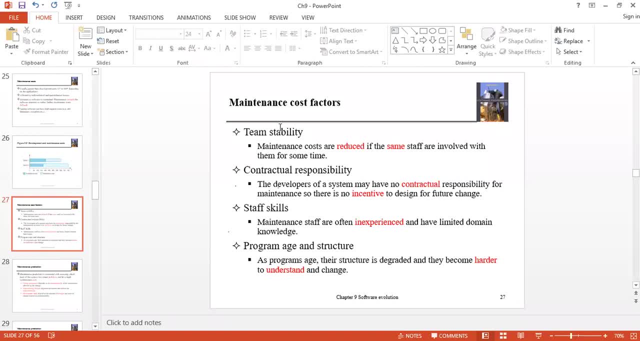 who has developed our software, the same team will maintain it. so we will have same team, same work we will have. so we have team stability is depending on it. we should have same team, ok, ok, ok, and you are understanding it. so it is easy to understand the program. 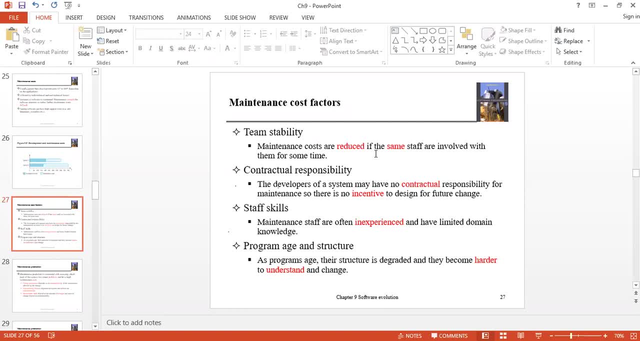 for it is understandable. ok, if it could be understand by itself and if it needs some modification. so you have to maintain this. you have to set a payment for The team that we hire. the developers of any system should be contractual based. If they are contractual based, then they will complete their work for maintenance. 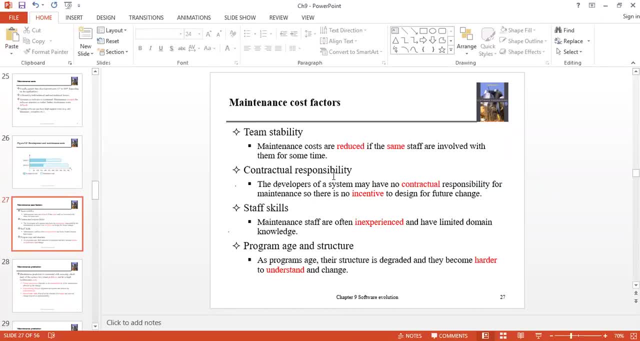 If we take responsibility for the maintenance, then they will come and do the maintenance every time. It will be an incentive part for us. Talking about staff skills, we have staff skills of any maintenance team. They have specifications in their own domain. They are limited. They have knowledge of their own domain. 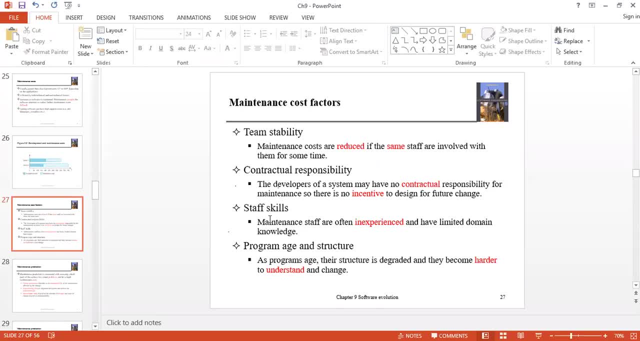 They are unexperienced for other domains. This is for the staff skills Program, age and structure. We will talk about the program age and structure. As much as our program is perfect, it will be old and aged. It will be difficult for us to understand. 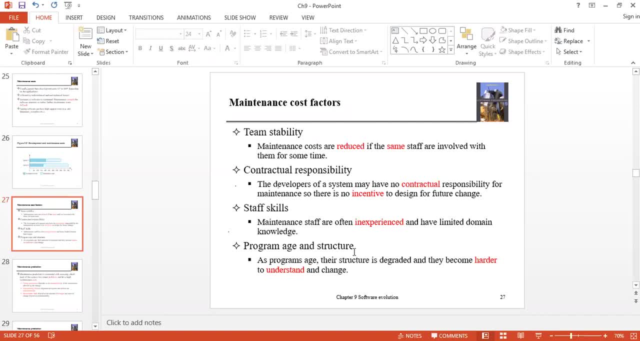 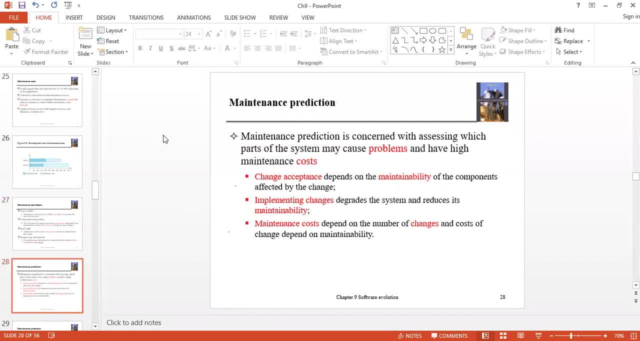 To make modifications in it. They are talking about this. These are 5-4 factors. Our maintenance cost depends on them. We have already read this point earlier. The cost is more on old programs as compared to new programs. We have a language barrier. 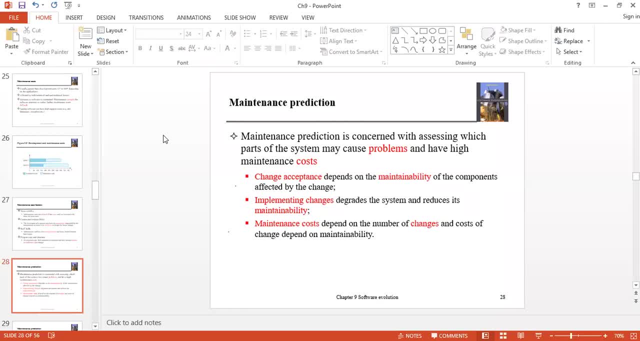 They use very old languages. They use old development and old compilers. They are not understandable for us today. If we apply maintenance on it, it will be difficult for us. Maintenance prediction. Here we have the predictions of maintenance. There is a maintenance prediction. 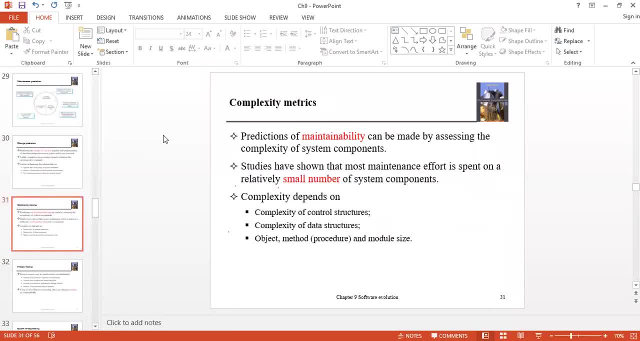 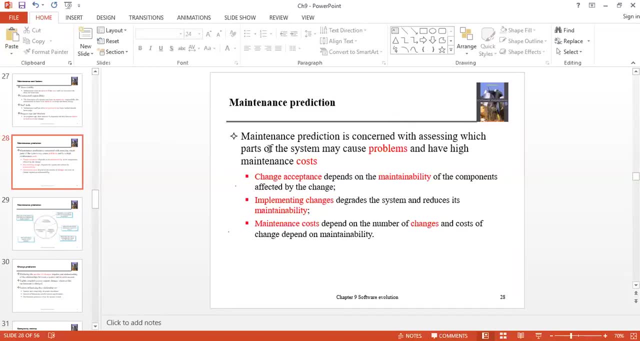 Then there is a change prediction And then we have all the complexity matters applied on it. What is the maintenance prediction? It is concerned with assessing which part of the system may cause problem and have high maintenance cost. What are we applying on the maintenance prediction? 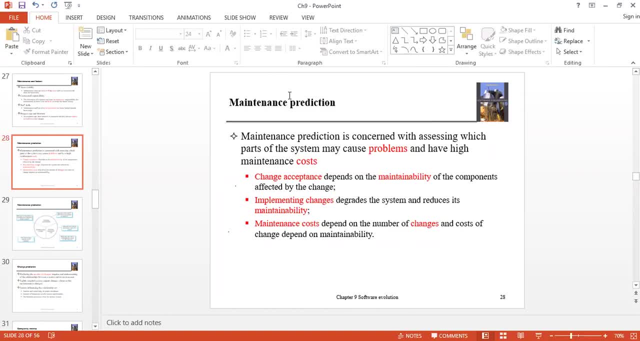 We are applying on the maintenance prediction: Which part of the system is causing the most problem And on which part will the cost be applied the most? We will look at these two things. For example, if your system is broken, Then you will look at those components. 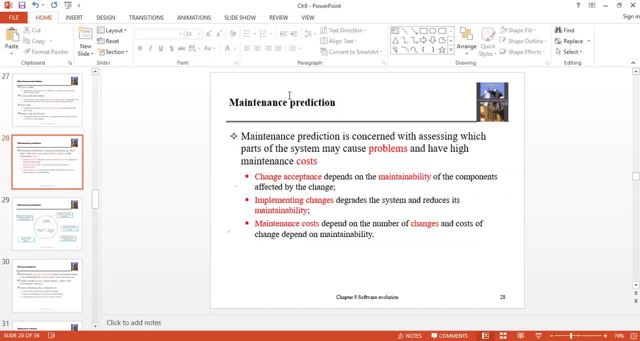 Which one is causing the most problem And if we come to fix it, Which one is causing the most problem? Which one is causing the most cost? Now they have told three points from this Change. acceptance depends on the maintainability of the components affected by the change. 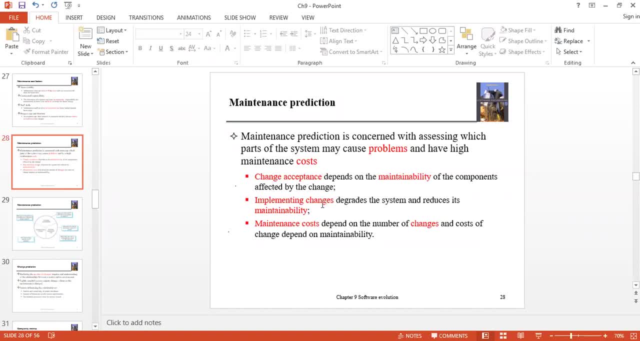 And on the second number, they are saying: implementing change Decrease the system and reduce its maintainability. Implementing change will happen, Change will happen. And then we have the maintenance cost. These are the three parts that we count in this prediction. 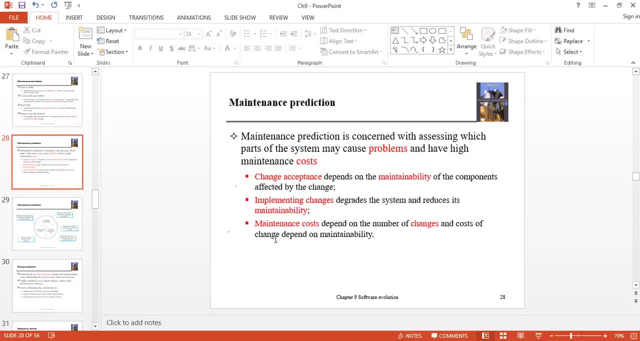 It depends on the number of changes And cost, And cost of change depends on maintainability. It is talking about cost, It is talking about implementation change And it is talking about change acceptance. We define it like this through the graph: How prediction, maintainability happened. 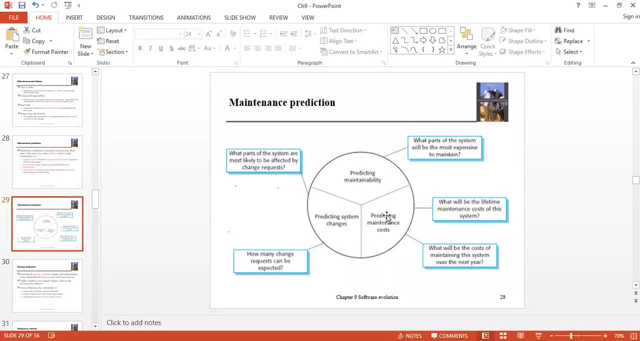 Prediction system changed And prediction maintenance cost. It depends on the wording that we have here, And by doing this you will be able to write in an understandable form: Prediction maintainability. What is it saying? It is saying what part of the system will be the most expensive to maintain. 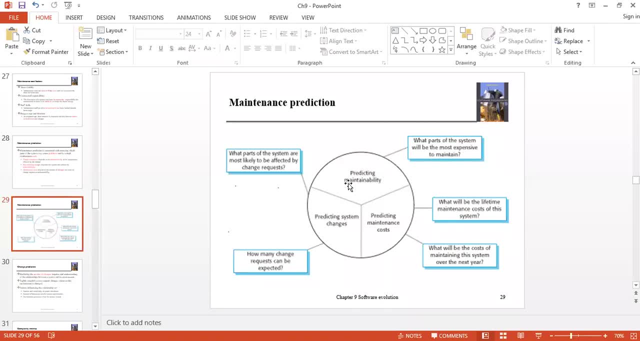 That is what we are seeing in the maintainability. What is the part that is the most expensive if we maintain it? Okay, Then if we look at this side, two questions are arising in this: In the prediction system change, where the system change is being talked about. 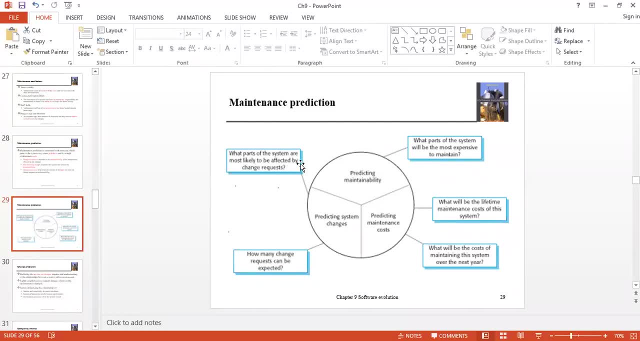 What part of the system are most likely to be affected by change request? What is the part that, if we request change, which part will be most affected? Okay, How many changing request can be affected, That is, how much change is expected in this system? 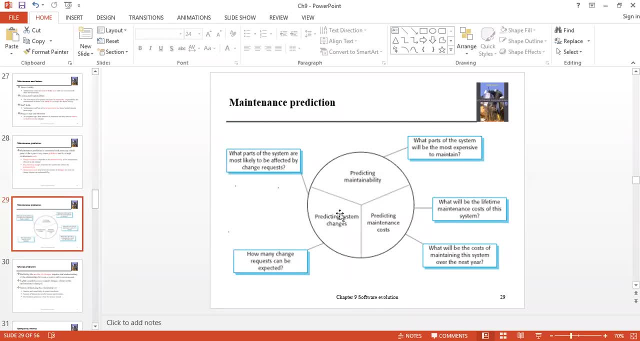 Which is required for us Multiple counting. It is asking: Okay, Then it is saying that it is talking about cost. It is talking about cost. What will be the lifetime maintenance cost of this system? That is, what is the lifetime cost?